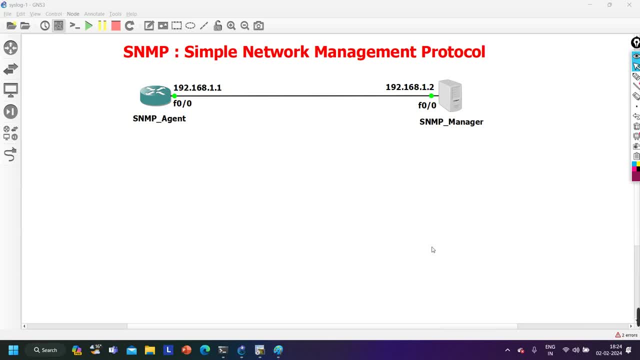 what is the deployment of SNMP, how to deploy SNMP in real time network. Then we will discuss types of messages in SNMP, like get message, set message and trap message. Then SNMP uses which protocol, like UDP or TCP. So it uses UDP protocol number. sorry, port number 161. 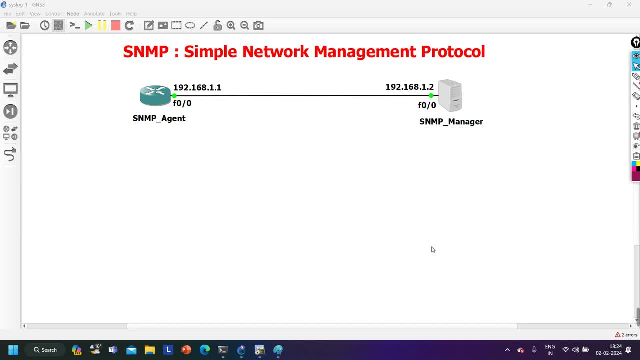 and 162. So you have to understand the scenario when it will use port number 161 and 162, because sometime interview is asking this question to you. know, engineers, like what? in what scenario SNMP client will use Port number 161 or 162, or SNMP manager will use port number 161 and 162. Then, guys, we 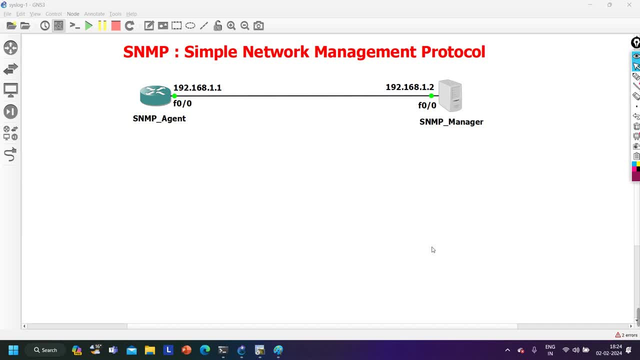 will understand the version: version 1,, version 2 and version 3.. What is the difference between version 1, version 2 and version 3.. Nowadays we are using, as SNMP, version 3.. So you have to understand the logic why we are using version 3, because anyone can ask you what is the benefit. 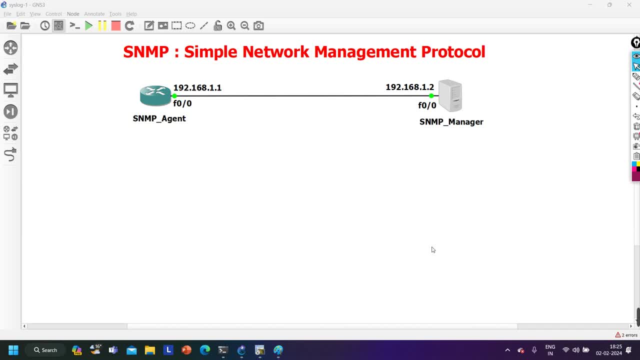 of SNMP version 3.. And then, finally, we will move to the configuration part: How to configure SNMP on Cisco routers and switches. So here you can see, this is my scenario. In my scenario, this is my SNMP manager, or you can say SNMP server. So there are two roles of devices. 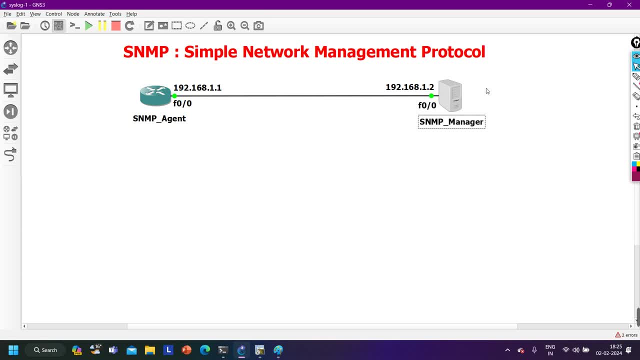 in SNMP, SNMP server or you can say SNMP manager, and another one is SNMP agent or you can say SNMP client. So here you can see, this is my SNMP server or SNMP manager, and this is SNMP client. So you can say SNMP server over here. but because you know, this is not in your syllabus as well. 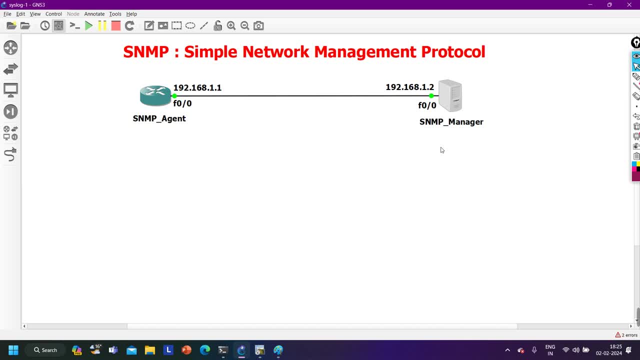 Like if you will check your CCNA, CCNP and CCI syllabus even right. You don't need to configure SNMP server. SNMP server is nothing but end machine. Like it can be your computer, it can be your windows servers with SNMP software. So to use a device as a SNMP manager or as 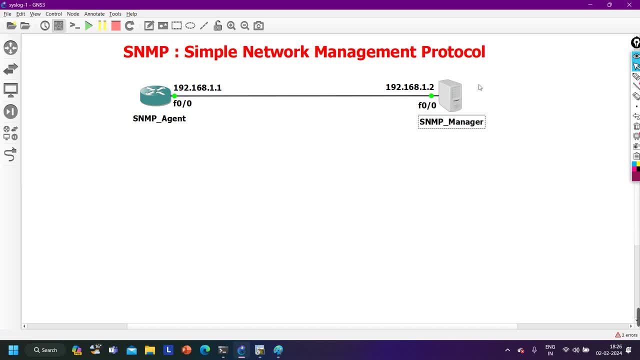 a SNMP server. you only need to install SNMP software there, Then that device will become SNMP server or SNMP. you can say manager, Your task is configure SNMP client. or you can say SNMP agent, like your routers and switches. Fine guys, so without wasting our time, let's begin. 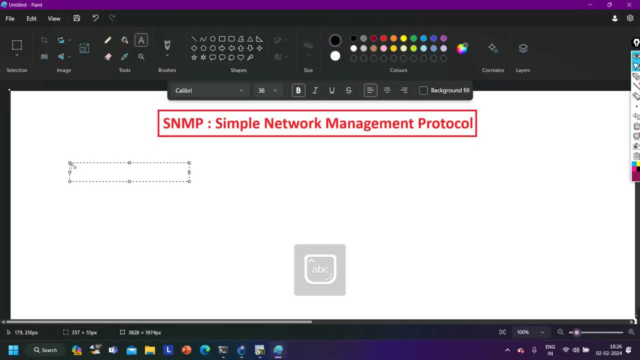 Now first try to understand why we need SNMP. Why SNMP? So, guys, let's understand. let's assume that I am a network engineer in a company and I have 200 devices in my network. What I am saying: I am a network engineer in a company and I have 200 devices in my network. I just 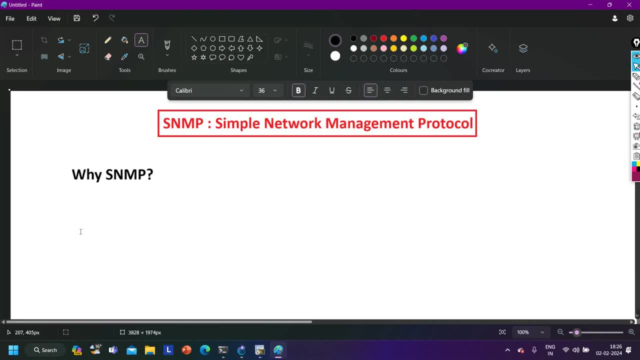 want to check which IIS version my routers are running, Which IIS version are running on the routers and you can say switches. So what option I have? First I have to access the devices. Again, I have two options: console access or remote access, but definitely in. 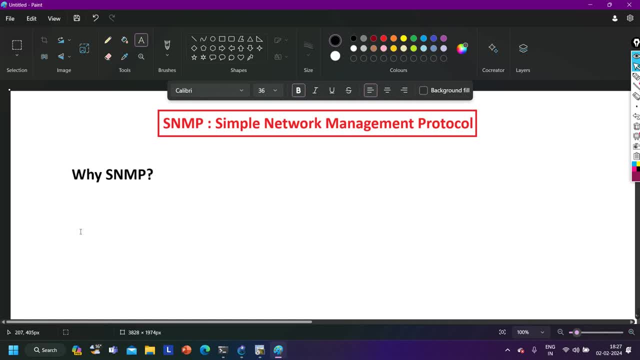 real time. you will have remote access. So let's say you have remote access and you have accessed the device and then you will run command what so version. then you will run command so version. So you have to access 200 devices And you have to run this command on 200 devices. Getting my point Right? so 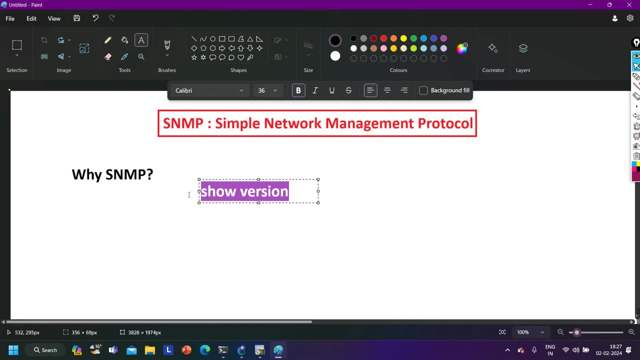 first I have to access 200 devices and then I have to run this command. so version Again, let's say it. I want to check IP address on a Router, 宅 router, let's say on r10 right, which is on second floor. i want to check ip address on fastethane. 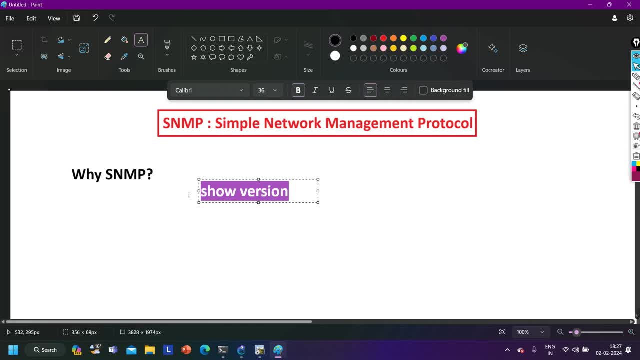 0, 0 of router 10. so first i i have to access router number 10, right, then i will run command. so ip interface: fastethane 0, 0. it will show me the ip address on fastethane 0, 0. let's say i want. 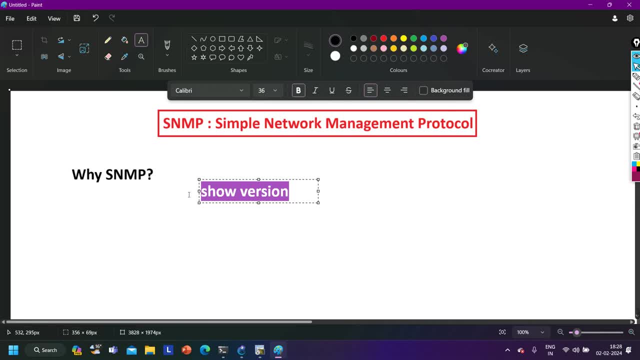 to check cpu: utilization of device, cpu selection of router number 20: again i have to access the device. i have to run command: show process processor, cpu- right. so this is first way. first way is first you have to access the device. you can access through console port or through remote. 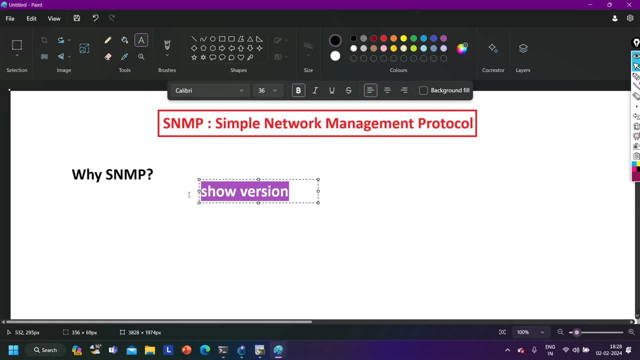 access and then you can run the command, whatever output you want. what is the second way? this is the first way and you all know this method. what is the second way? the second way is protocol. second way is protocol, and that protocol will give me information, right, like i want to know. the is version of a device, right, so i will run a. 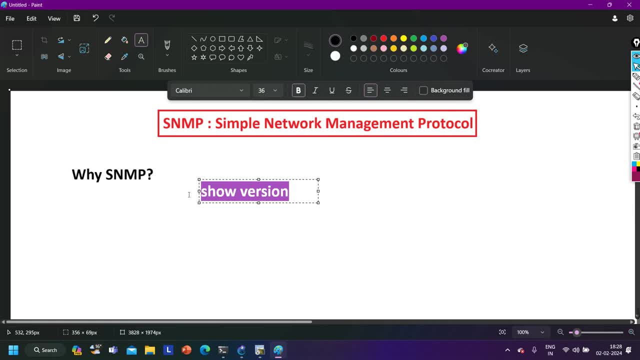 protocol and that protocol will be responsible to provide me the is version of devices. getting my point. and that protocol is snmp, simple network management protocol. why we are saying simple network management? because here you will get gui access right. so gui is simple. that's why we are. 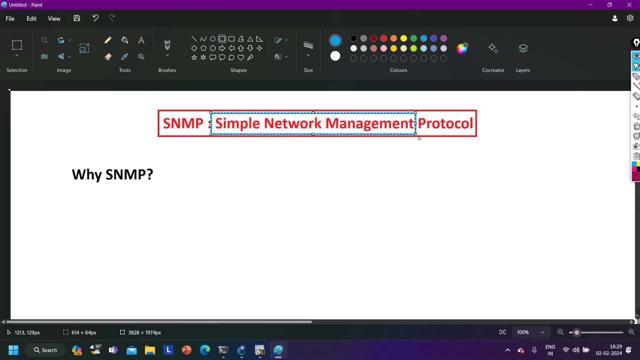 saying it is simple network management protocol protocol- fine. so through snmp protocol we can gather the information of devices or we can configure the devices as well. let's say we have 200 devices in my company and i want to create one access control list. so again, i have to first access the device and then i can configure. 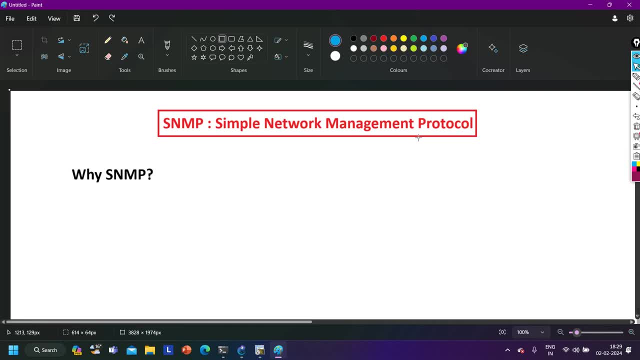 access list there, right, but through snmp. this is first option. second option is snmp. through snmp also you can set hostname right, acl on the devices with the help of one command, that is, you know, in the snmp messages you are going to understand, there is one set message. so simply on snmp server. 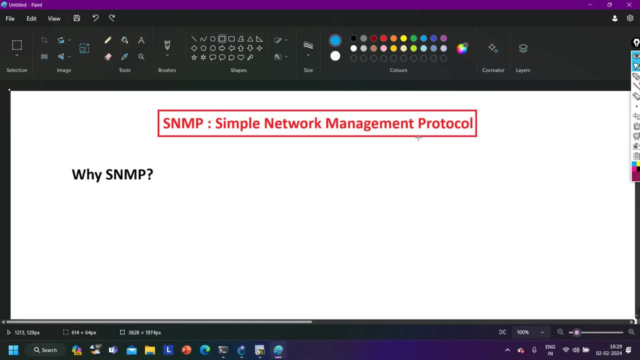 you will provide the target ip address, ip address of your device, and then you will send you know set message, set hostname r1 right and your snmp protocol will put push that command to router, right to snmp client or snmp agent. you can say: then device will automatically configure ip address on interface or we. they can change the. 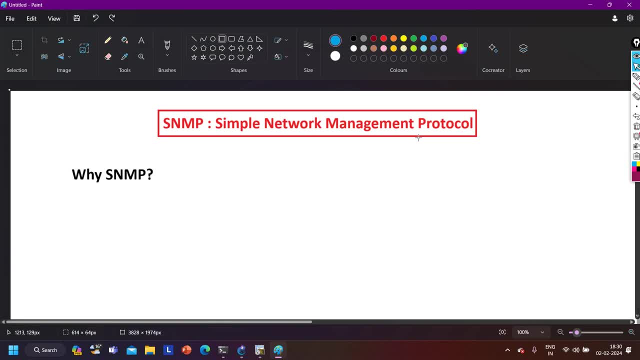 host name. getting my point, in the same way we can configure acl, also any configuration. so you already know the first way. first way is very simple: manually you can access the device and then you can configure the device right or you can gather the information. the second way is: 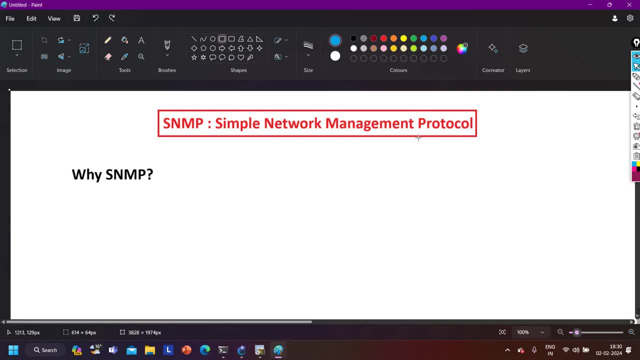 protocol and that protocol is called snmp protocol. so hope not this is kill. this part is clear to you, like why we need snmp guys? because in snmp we have a centralized device. from a centralized device or from a centralized location, i can configure the devices, i can gather the information or i can manage the devices. 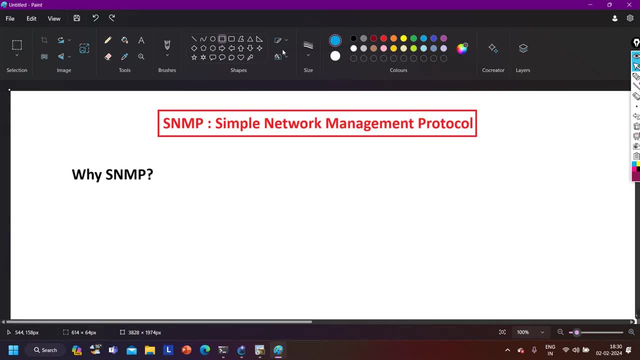 getting my point. let's say, i want to tell my device. let's say, this is my router. i want to tell my router: brother, whenever your cpu utilization will reach to 80 percent, please send me a log message. right, your device will send a log message to your snmp server whenever. 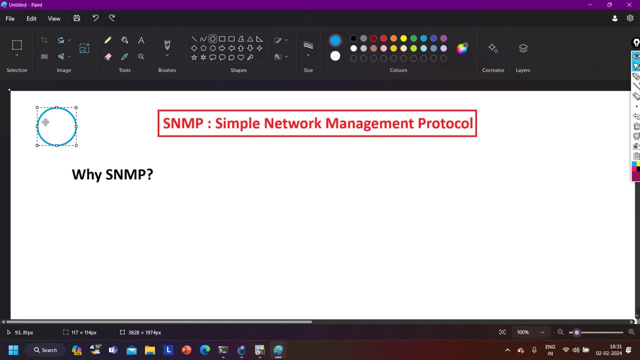 cpu utilization of your device will reach to 80 percent, right? so these are the reason why we are using snmp guys in real time. fine, now to understand how snmp works, first you have to understand the roles defined in snmp deployment, roles of devices in snmp deployment. 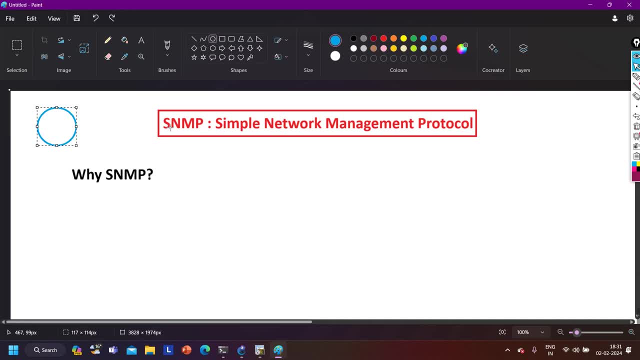 so, as i told you, there are two types of roles in snmp. first one is snmp, let me write here. first one is snmp agent, or you can say client- snmp is few people are saying client, few are saying agent. and second one is snmp manager. 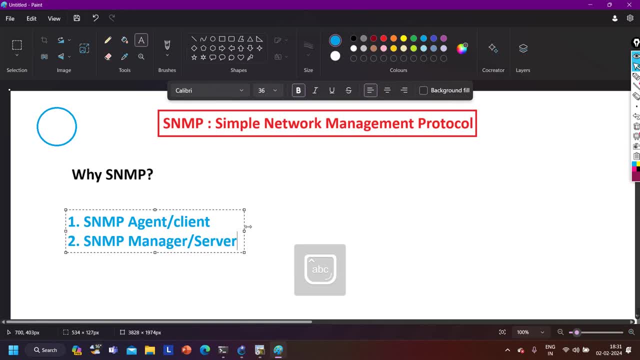 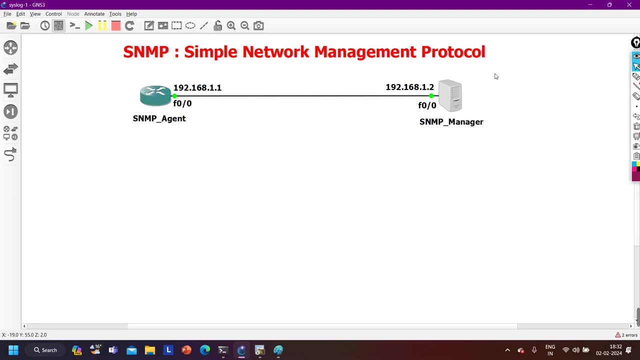 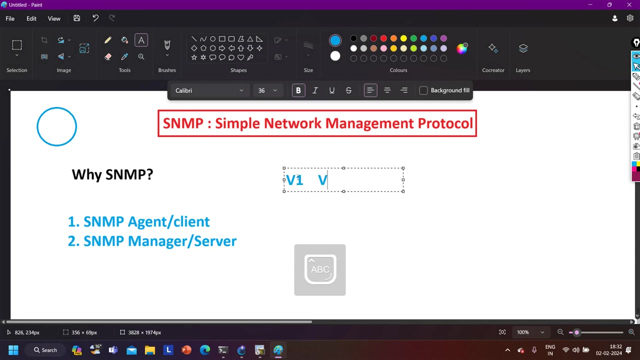 manager, or you can say what snmp server. fine, so in this scenario, you can see in my topology again, i have one snmp client and i have one snmp server. you can say: this is snmp manager, this is snmp agent. right now, guys, in snmp we have three versions: right version one, version one, then we have version. 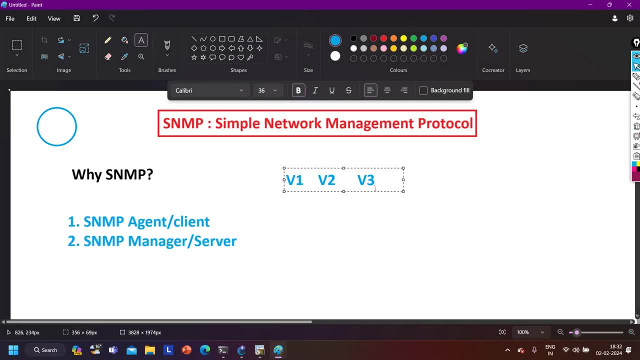 two, and then we have version three. right nowadays we are using version three because version three is secure right. soon we are going to understand this version right in detail: version one, version two, but for now what i am saying: in version one we have some messages. in version one we have some. 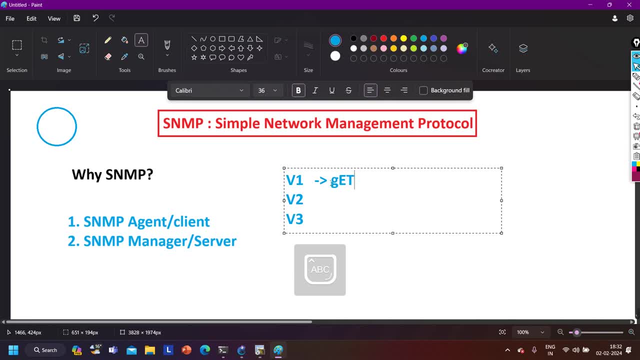 messages like set message. or you can say: first message is get message, get message. then we have set message. i'm going to make you understand the meaning of each message, don't worry. right, set, get message, set message. and then we have one trap message, trap message. right in version two, again, we have three messages. 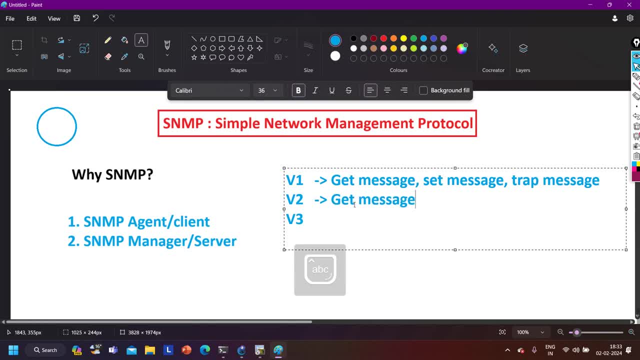 get message, get message, set message and inform message. in for message. again in version three also, we have these three types of messages: get message, set message and inform message. Then if you are thinking what is difference between version 1, version 2 and version 3? because there is one different difference in version 1 and version 2, that is, in version 1 we have trap message. in version 2 and 3 we have informed message. right, 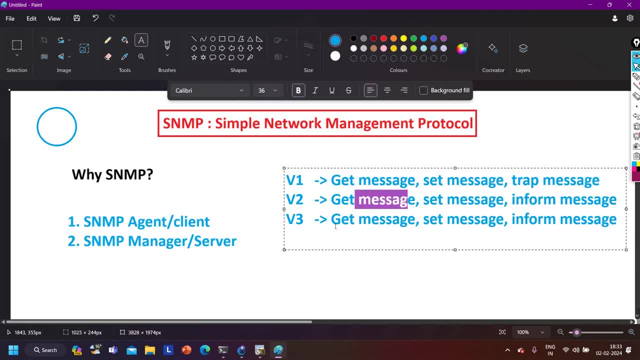 Then what is the difference between version 2 and version 3, guys? version 3 is secure, version 2 is not secure, right? communication will happen in plain text in version 1- sorry- in version 2, and here communication will happen in cypher text in version 3. so we have authentication. we will discuss about that authentication also, right? 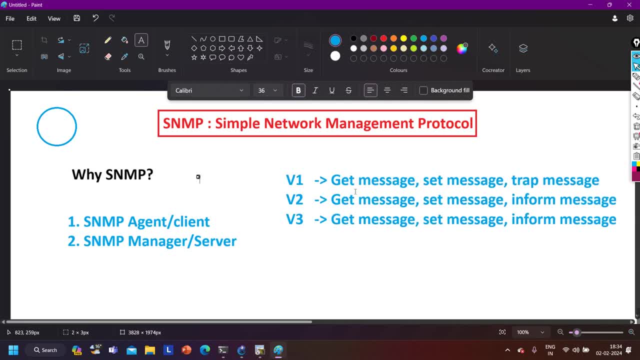 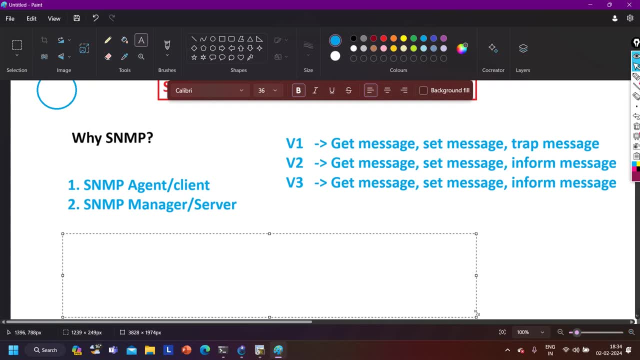 Now try to understand these messages. first, what is the use of get message right? first let me give you one overview of these messages. after that, If it Will be quiet, I will discuss. you know the details, information as well, about these messages. first, messages get a message, so guys get a message is used, it is used to retrieve information. information from SNMP isn't, isn't or you can say: 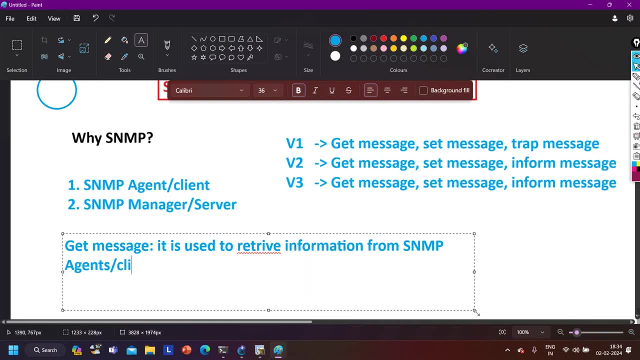 What clients, Clients, Okay, SNMP get message is used to retrieve. or you can say: gather right, gather the information about SNMP client or SNMP isn't Fine, Hope it this is clear to you. like, let me give you some example as well. like I can say what: get me, get me hostname, get me hostname. then I can say: get me interface IP address, interface IP. then what I can say: get me information about ERP protocol, get me information about OSPF protocol, get me CPU utilization, get me IOS version right. so these are examples. 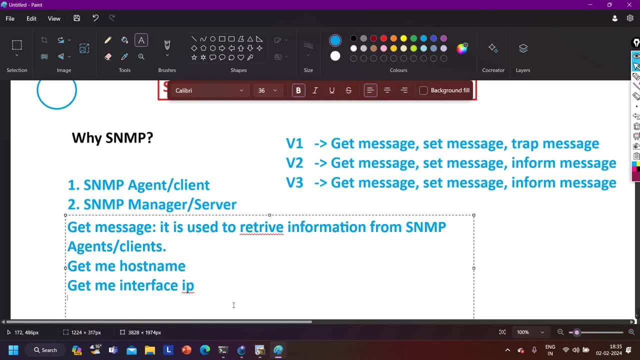 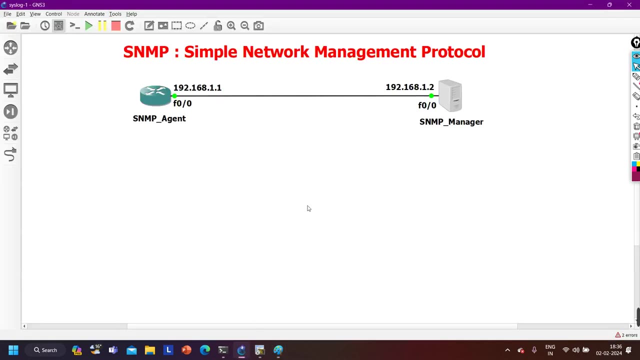 Right Of get message. so through get message, we will retrieve the information from SNMP client to SNMP manager or SNMP server, right? So let's say, in this scenario, in this scenario, from the SNMP server, I want to know what I use version is running on this router, right? so this is my SNMP agent, this is a SNMP server or SNMP manager. so from SNMP manager I will send which message. 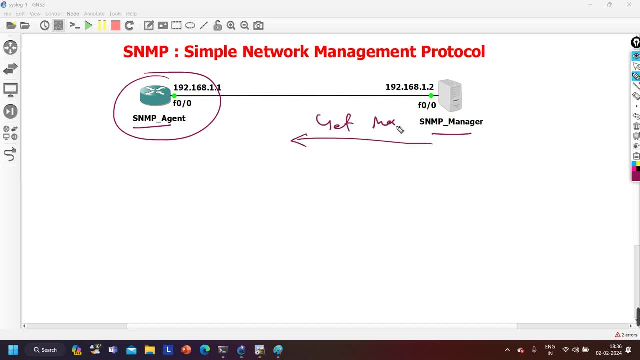 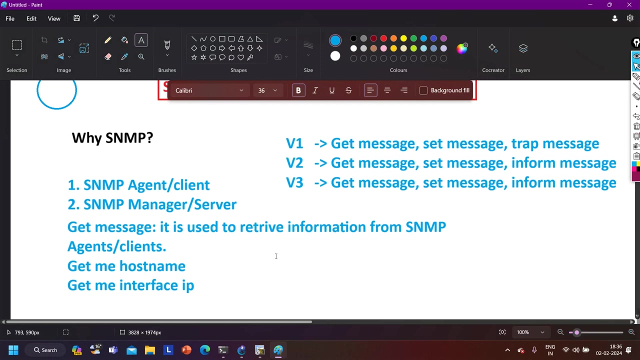 I will send get message, Get message Right, and here we will say what get me? get me hostname, Hostname. Getting my point. so this is use of get message. get message is used to retrieve the information of SNMP agent. fine, hope this is clear now. next message is set message. 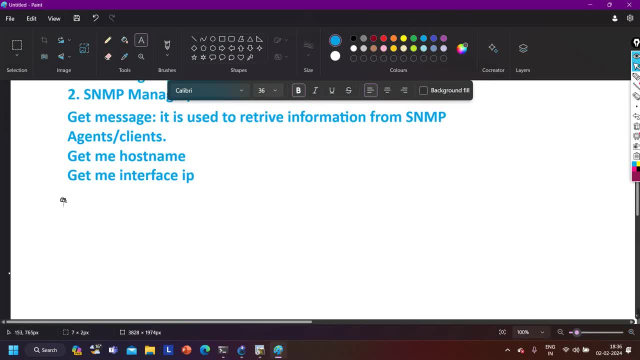 Set message. Let me write the small definition of set message as well here. and you know one more thing about get message. I'll just keep in mind this is important point: get message. message is always forwarded by Manager, Getting tracked By Manager. 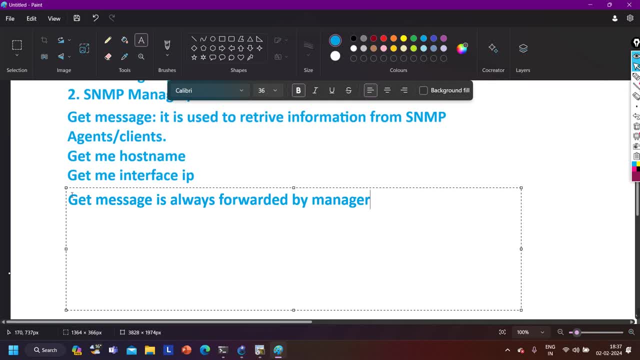 Get message is always for worldwide SNMP manager: Snmp. Snmp is an Application here protocol. It is an application layer protocol. ачеuki siya. It is an Application Layer Protocol Protocol protocol. Application Protocol layer protocol. 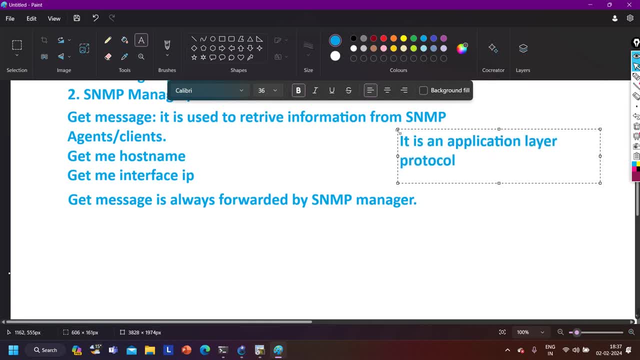 Protocol, Protocol Protocol. fine means this protocol works at application layer. all messages of snmp will be generated at which layer guys. at application layer, again, all the application layer protocol will use either tcp or udp at transport layer. so it uses. it uses udp port number, port number 161 and 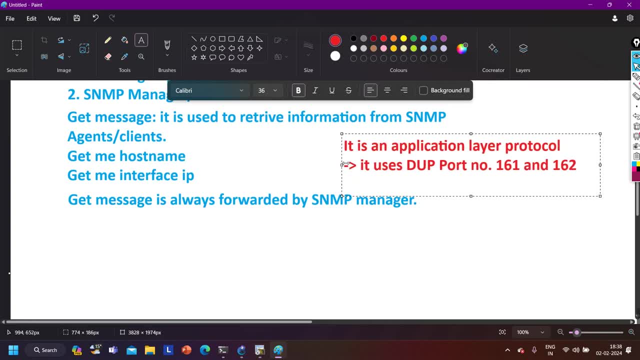 162. right, these are two basic points about snmp protocols. so always keep in mind it is an application layer protocol which uses udp port number 161 and 162 and get message: get message. as i told you, get message is always forwarded by snmp manager and manager will. 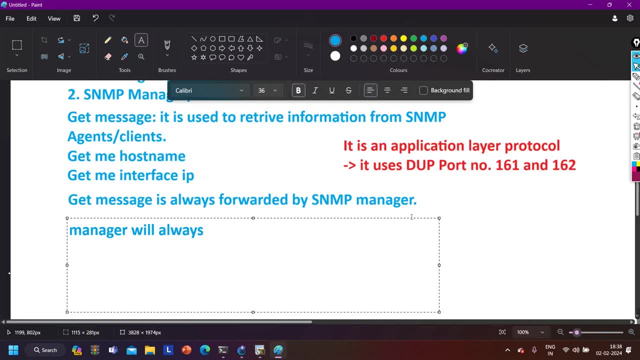 always, always use port number 161. right manager will always use port number 161 for get message. message for get message. now. hope this is clear to you. get message is clear to you. fine, now let me move to set message. set message. next message is set. message set. 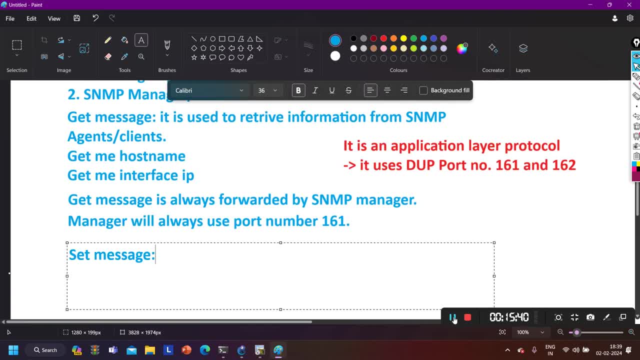 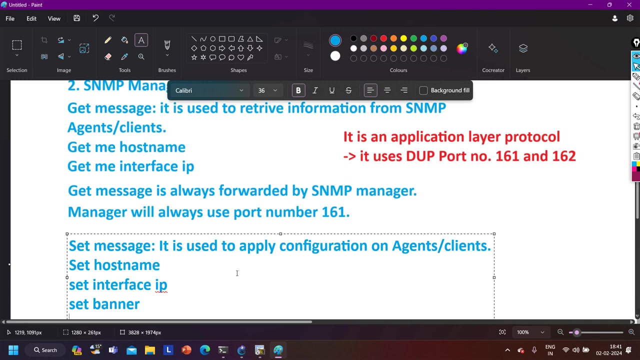 message. so see, guys, set message is used to used to apply configuration on agent, on sm, snmp agent. so what we can say it is it is the friends settings of clients get message to get message of guests out. set interface, IP interface, IP set banner. get me a point. these are what example of? 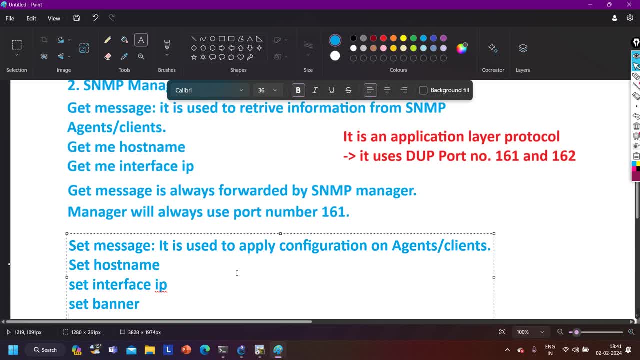 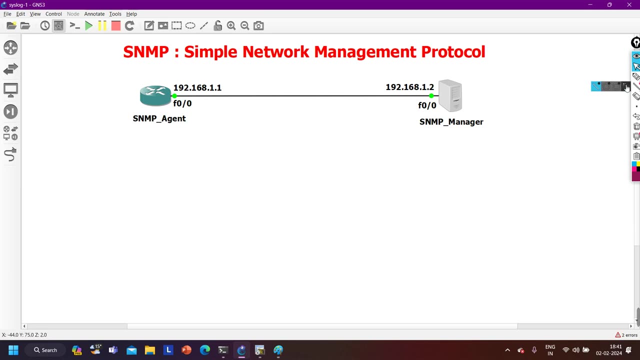 set message. so if you want to configure anything on device, you will use which message set message. again, set message will be forwarded by SNMP manager. always right manager will always forward this message set message. so here, in this scenario, let's say I want to configure hostname on this agent device, right on. 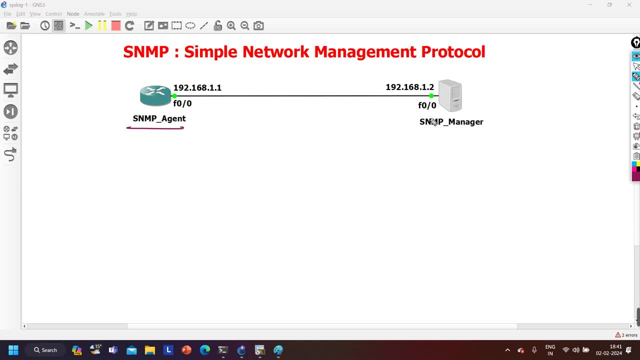 SNMP agent, from SNMP manager, from SNMP server. so what I will do from here? I will set, send one set message, set message, right. and set message is what? set hostname, let's say R1, right. so once this agent or client will receive the set message, it will set their host name, R1, right. 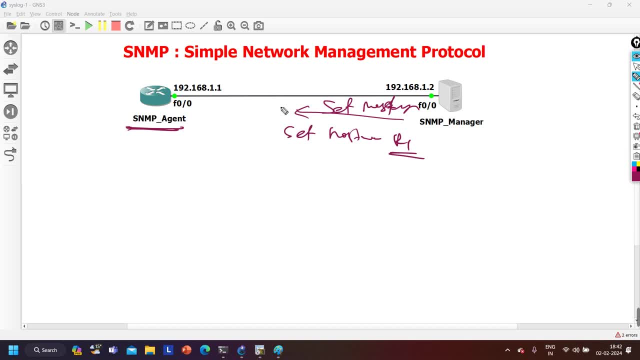 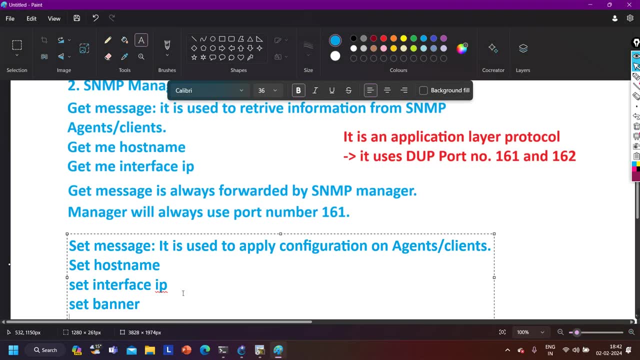 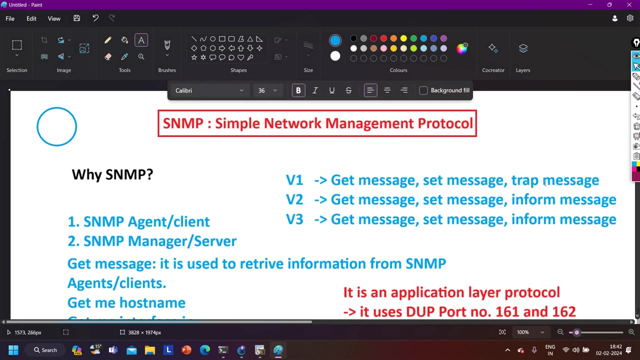 from the default host name. get me a point, fine. so hope now set message is also clear to you. like this you can assume multiple examples right. find now next message is: what trap message? trap message, and then we will discuss the informed message. right? so next message is trap message. first, let 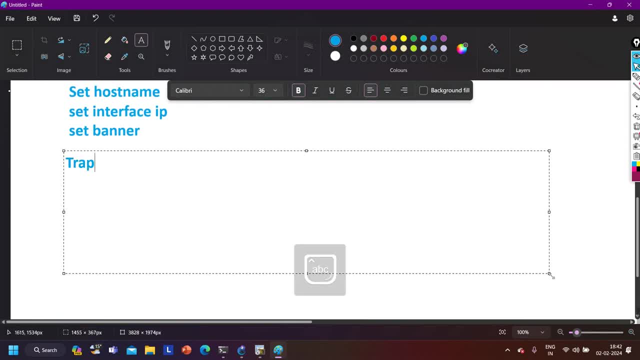 me discuss about the trap message guys. trap message, trap message. it is used for condition. what I am saying? it is used for condition and this message will be always forwarded by agent. condition means what condition means? let's say, I have configured my device in such a way so that my device will generate one. you know, log message. 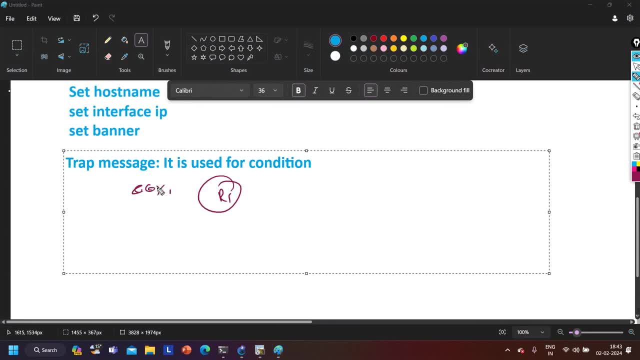 whenever CPU utilization will reach to 80 percent or when temperature will reach to 40 degree Celsius. let's say I have defined this condition on R1, then whenever your temperature will reach to 40 degree Celsius or your CPU utilization will reach to 80 percent, please. 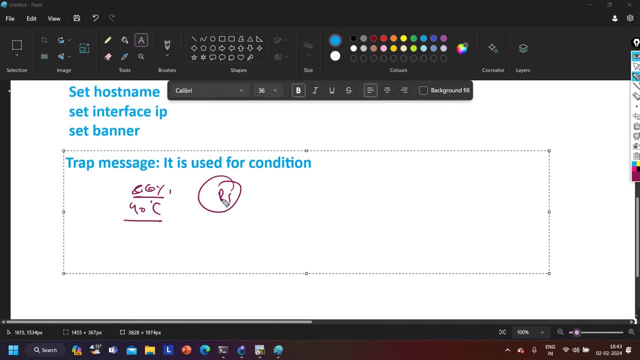 generate a syslog message, right. so, whenever temperature will reach to 40 degree Celsius or CPU utilization will reach to 80 percent, It will give me one log message. it will generate one log message for SNMP manager and it will send that log message. with the help of what trap message? with the help of trap message. 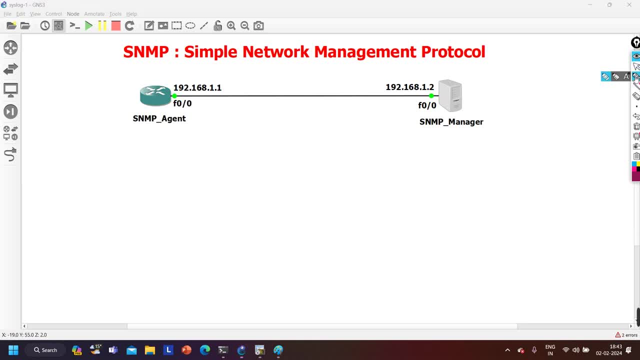 so, again in this scenario, let's say I have configured this router to generate a log message- syslog message- when CPU utilization will reach to 80 percent or when temperature will reach to 40 degree Celsius. right? so if CPU utilization of this device will reach to 80 percent, it. 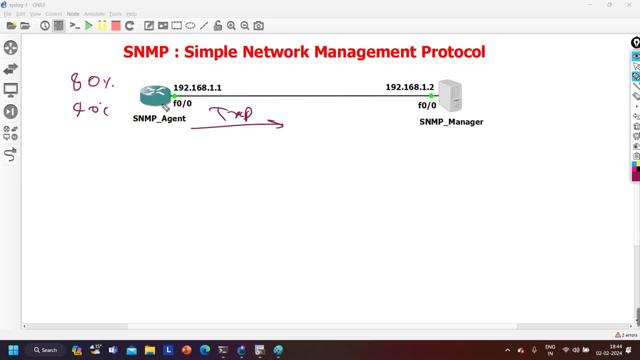 will generate a trap message. Or if temperature of this device will reach to 40 degree Celsius, again it will generate one trap message. right, so trap message will be forwarded by SNMP client or SNMP agent. you can say always right, and guys agent will send trap message on UDP port number 162, right. 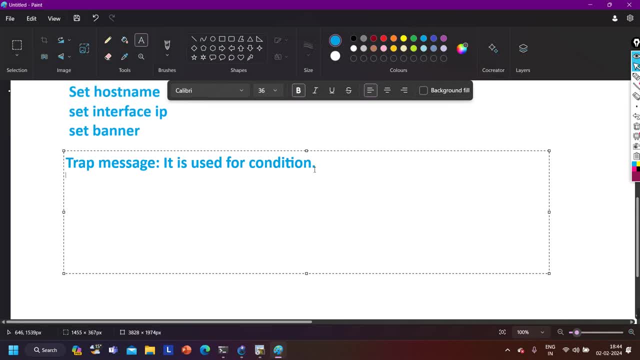 on port number 162. so now hope this is clear to you, like when we are using port number 161 in SS, SNMP and when we are using port number 162 in SNMP. so port number 161 will be used by SNMP manager to send, set message and get message, and port number 162 will be used by by SNMP. 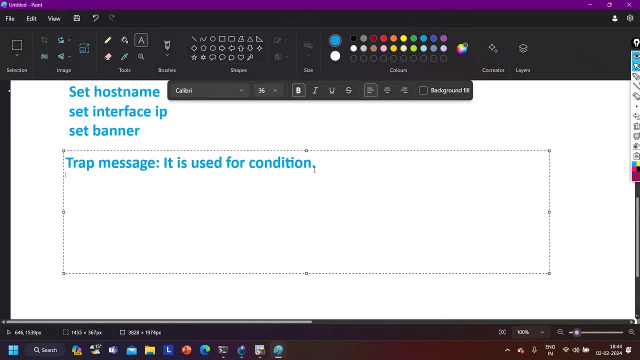 agent to see to send trap message. to send trap message. it is always forwarded by SNMP agent, SNMP client or agents right on port number 162. on port number 162, getting my point? so I have achieved any kind of condition through SNMP, like if CPU utilization reach reaches. 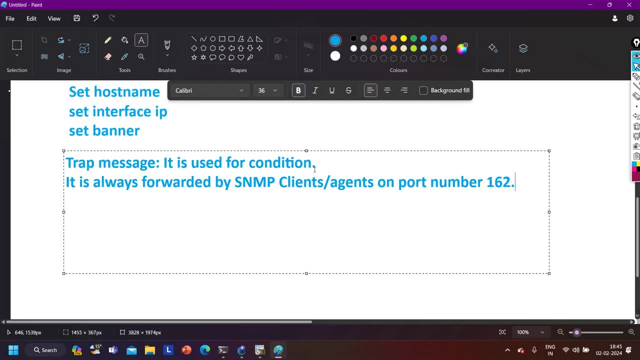 to 80 percent, Then generator syslog message. if temperature is more than 40 degree Celsius, then generator syslog message. all the condition message will be forwarded through port number 162 for management message. it uses port number what 161 like set message and get message. okay, guys. so if 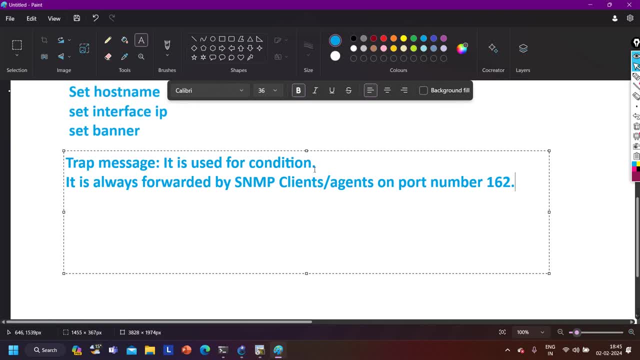 someone will ask you what is get message in SNMP so you can say this is one kind of read message. Through get message we are getting what only information. we can read it. we can check what IOS version is running, what IP address is running at, what is the banner on router, what is the. 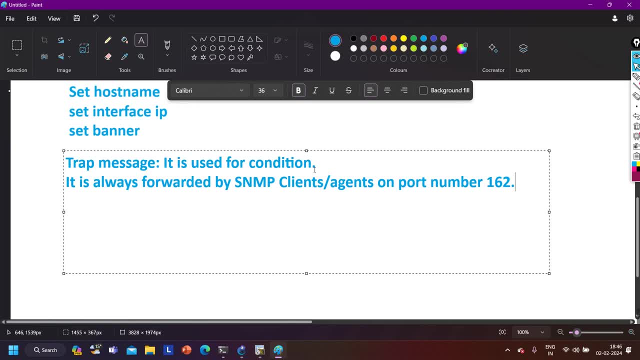 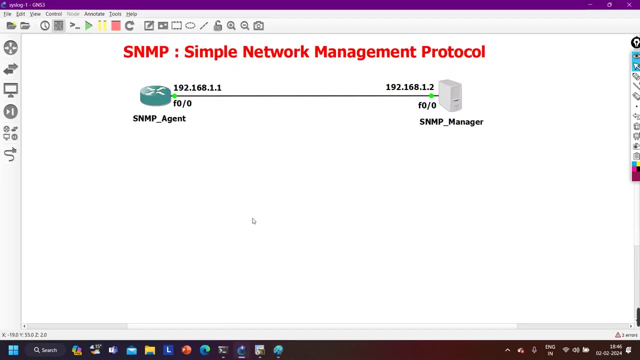 host name on router right. so this is a kind of read message: right, get message will be forwarded by SNMP server always or manager always. it is used to retrieve the information from client, right? so let's say, in this scenario, In this scenario, In this scenario, 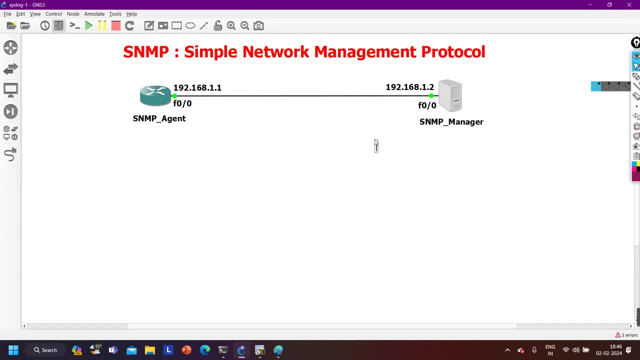 If server is going to generate one set message or get message, get message. what will be the information? guys, right, this is set message at application layer. at application layer, then at transport layer, what will be the information source port? source port will be any random port number. 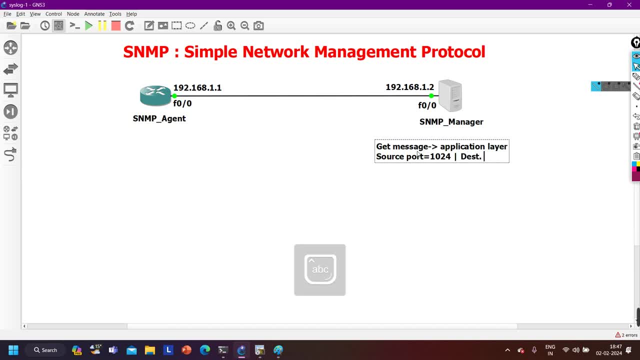 Then source IP and then destination port. destination port will be what 161 after that source IP. source IP will be the IP address of IP address of server SNMP manager, that is 192.168.1.2, and then destination IP. destination IP will be what the IP address of agent 192.168.1.2 will. 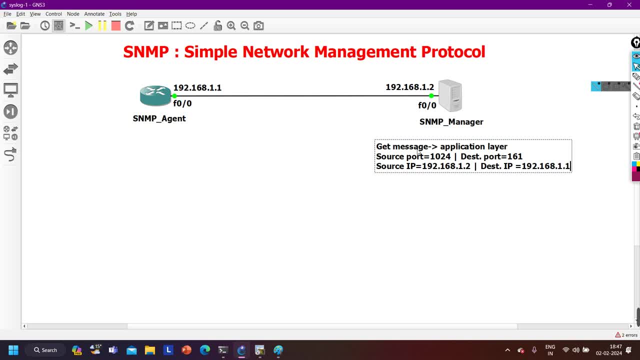 be what a destination? IP 192.168.1.1. who will provide the ip address of agent? you. you will define. the ip address of agent means target ip address, getting my point. then after that there will be layer 2 header. layer 2 header header getting my point. so this is how your set message get. message look likes: 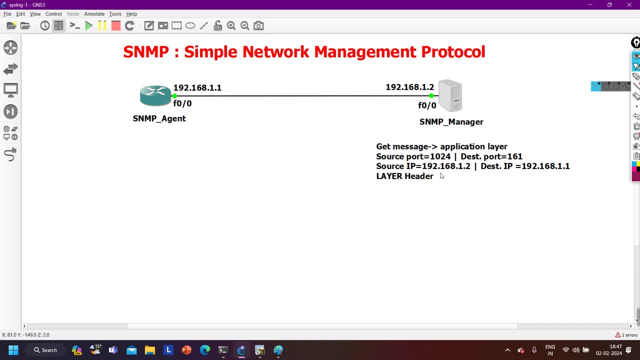 fine, so now hope this is clear to you, right? fine, then server will forward it to client means agent. fine again. in the same way, set message will look like at application layer. it will generate set message right to change the information on client or to apply the configuration. 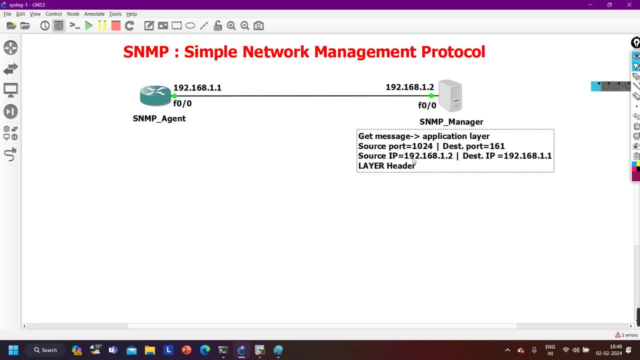 on client. you can say: getting my point, okay, so now let me move further. next is trap message. so see, let's say here i have defined one condition, that it uh condition is if my cpu utilization is to 80 percent and log message right. so if cpu utilization of this device will reach to 80 percent, this device will. 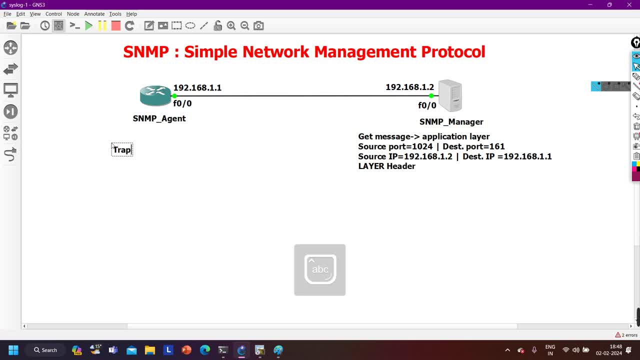 generate bait. what one trap message trap message at application layer. in the trap message again at layer four, it will use udp port number. what source port number will be the random port number? destination port will be 162.. destination port will be 162 under the trap message information. 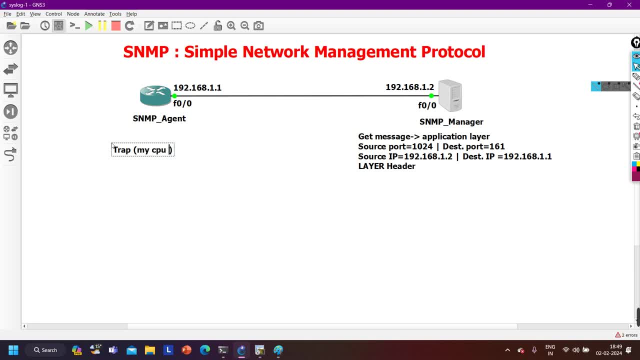 bit will be what my cpu is: 80 percent right. then there will be udp header, then there will be ip header and there then there will be Ethernet header. like this it will work right now. guys, you know, trap message is not reliable message. let's say this: 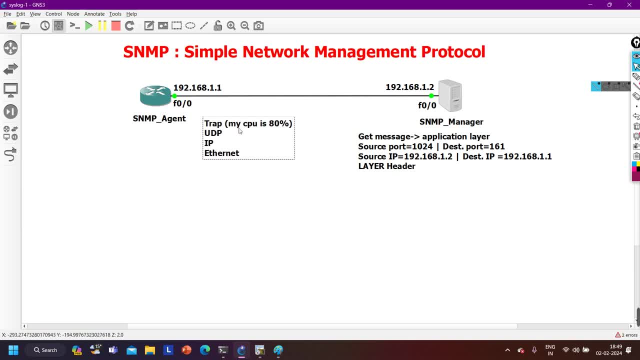 agent machine. agent device have sent this trap message to SNMP server, right, but because of congestion on the link, let's say server have not received this trap message right, so there is no any acknowledgement. so client machine will will never get to know that server you have received this message or not. server. 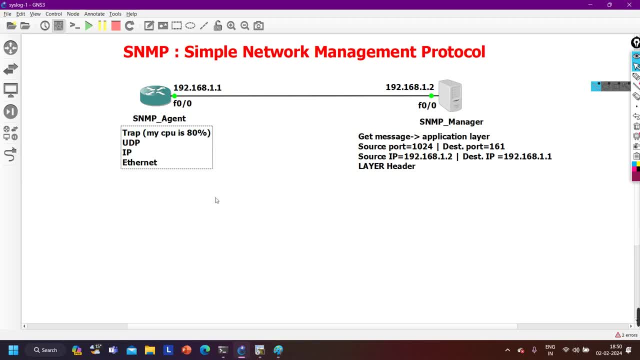 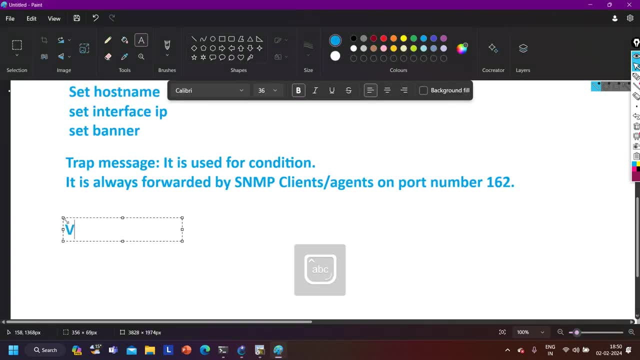 have received this message or not. so that's why we come up with SNMP version 2. this is all about SNMP version 1, so now hope SNMP version 1 is clear to you. in version 1 we have three messages: set message, get message and trap message. and 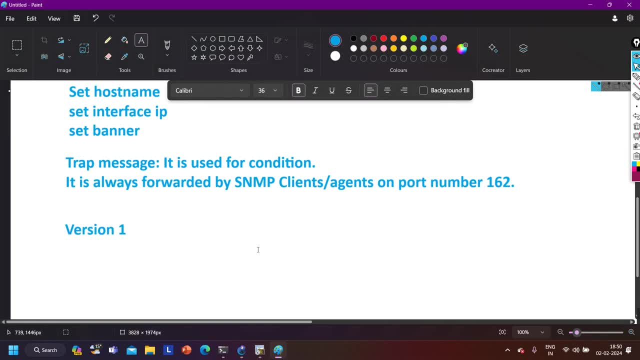 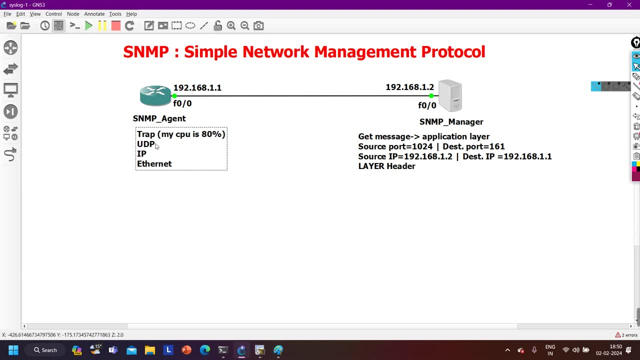 problem is trap message is not a reliable message. so if CPU transaction of device will reach to 80% it will generate a trap message for manager. but if manager will not receive it right, client will never get to know about it that my server have received this information or not. so that's why we introduce SNMP version 2. 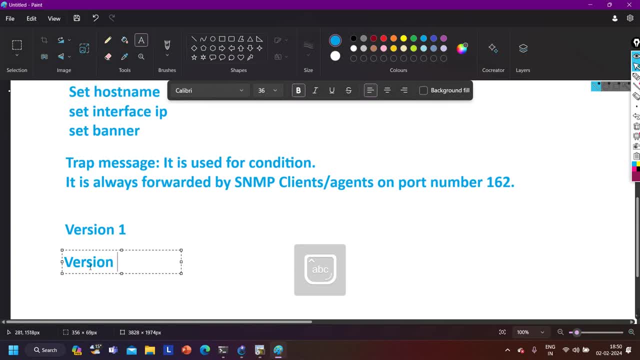 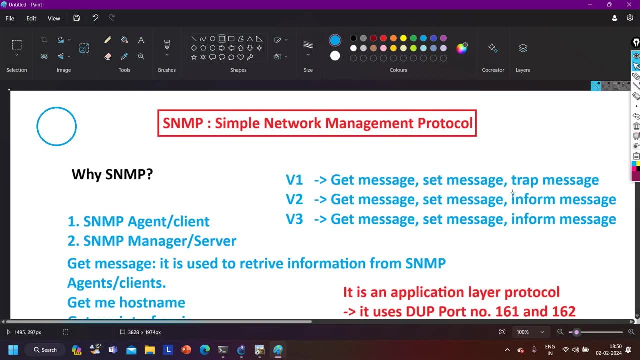 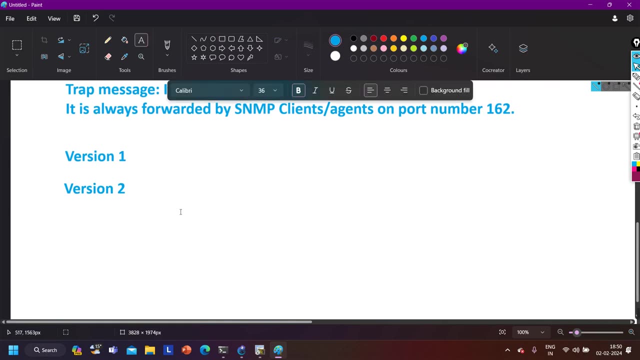 in SNMP version 2 we have which message guys? informed message, right. see, here in SNMP version 2 we have this message: informed message, right. so what is informed message? informed message is nothing but trapped message plus acknowledgement. trapped message plus acknowledgement. informed messages are poles information for active feedback. 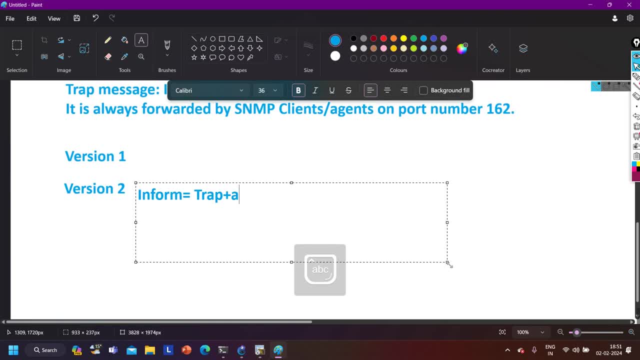 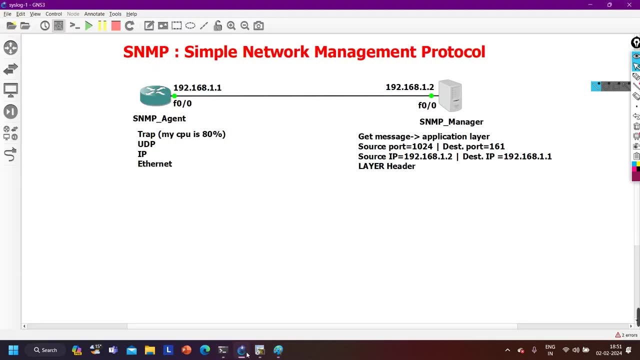 in farm messages equal to mute report: uterus babysitter trapped message. trapped message: inform message. in version 2: inform message it's saying my cpu is 80 percent. then it will forward to server and, as inform message is reliable, right when server will receive inform message it will. 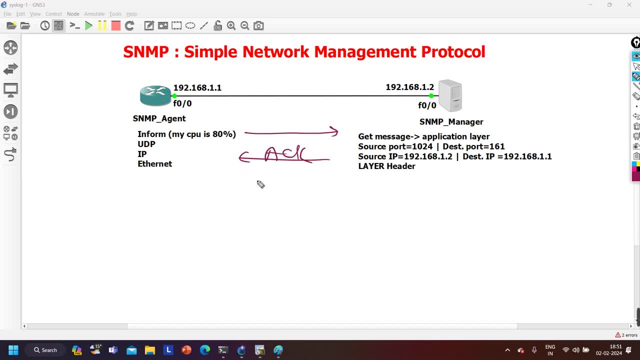 send what acknowledgement acknowledgement. so this is the difference between version 1 and version 2. in version 2 we introduce the new message that is, inform message and inform message, nothing but trap message plus acknowledgement means snmp server or snmp manager will give acknowledgement to client after receiving trap message. so that's why we come up with snmp version 2, again in snmp. 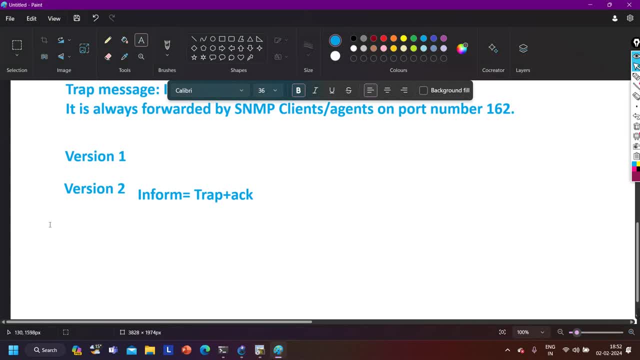 version 2. we introduce a new command. we introduce a new command. that command is that command is this: get bulk like in version 1- usb you have, or in version 2 you have. what message? get message right through. get message. what information you can gather. you can gather information of is version or ip address on: 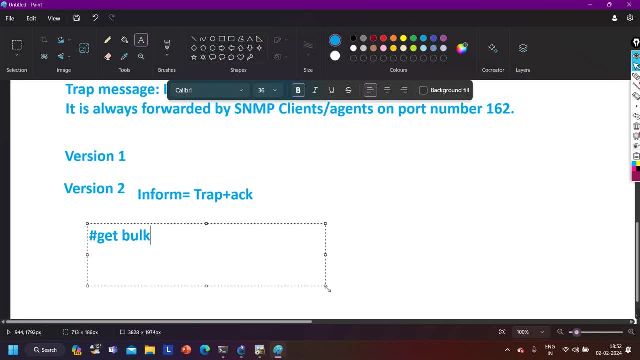 interface right host name. this is not detailed information. but in version 2 we have a new message that is get bulk. so you can run this command in version 2, get bulk, to gather the detailed information. like in version 1 you have this message: get message and you have said get me, get. you are sending get, get message to get the ip address, interface ip address, interface ip. so client will send you the ip address on the interface. but in version 2 you you have what message: get bulk. so if you will set get bulk right and then interface ip, so client will send you the ip address on the interface. but in version 2 you you have what message get bulk. so if you will set get bulk right and then interface ip, so client will send you the ip address on the interface. but in version 2 you you have what message get bulk. so if you will set get bulk right and then interface ip, so client will send you the ip address on the interface. but in version 2 you you have what message get bulk. so if you will set get bulk right and then interface ip, so client will send you the ip address on the interface. but in version 2 you you have what message get bulk. so if you will set get bulk right and then interface ip, so client will send you the ip address on the interface, but in version 2 you you have what message get bulk. 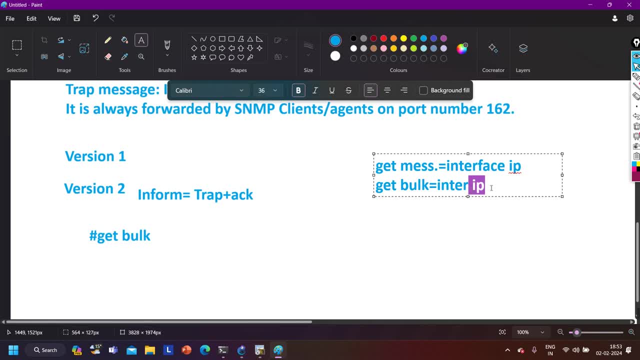 definitely it will give you the ip address of interface. apart from it, it will share more information, detail information like mtu, speed, bandwidth, submit, mask the many more information right. so, guys, the difference between get message and bulk message is what get message will give you particular information and get bulk message will give you the detail information right. get bulk will give you detail information like ip address. 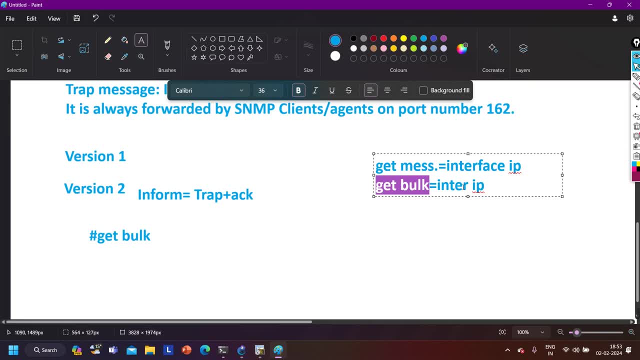 the mac address of interface: mtu crc packet- right and many more information. the mac address of interface: mtu crc packet- right and many more information. the mac address of interface: mtu crc packet- right and many more information. right, but version 1 and version 2 are not secure. right, but version 1 and version 2 are not secure. right, but version 1 and version 2 are not secure. right because in version 1 and version 2. right because in version 1 and version 2. right because in version 1 and version 2, your packet will travel in plain text. your packet will travel in plain text. your packet will travel in plain text, plain text. so that's why we introduced plain text. so that's why we introduced plain text. so that's why we introduced version version. 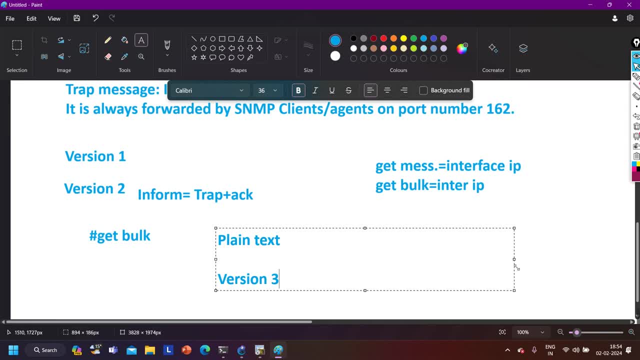 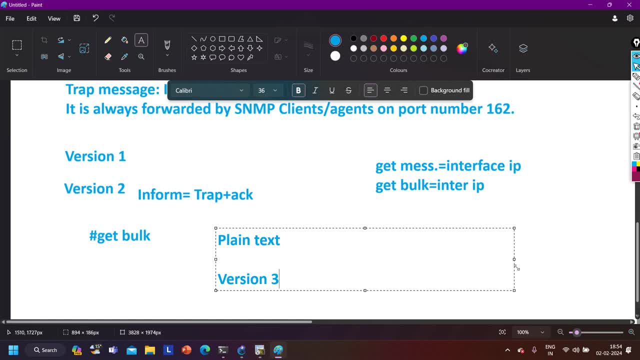 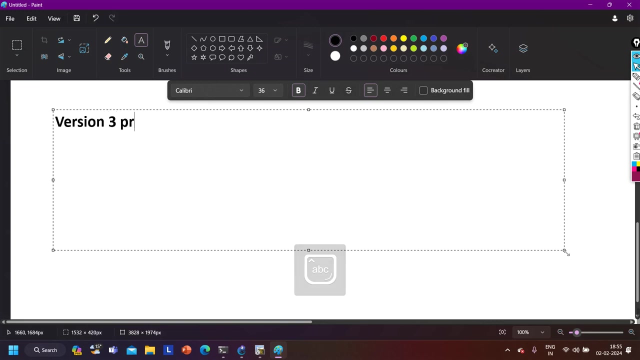 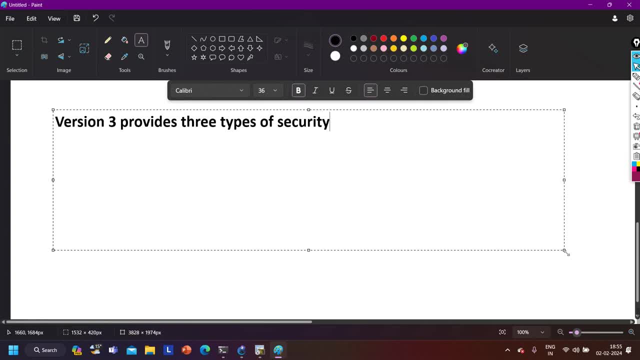 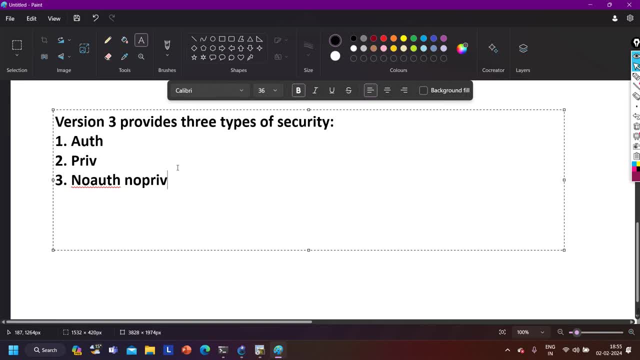 But if you want to configure authentication security, so you have option right. Auth means authentication, Auth means authentication. right, Like here, we will define the key. We can define key. Priv means what? Priv means guys, privacy, Privacy means encryption. 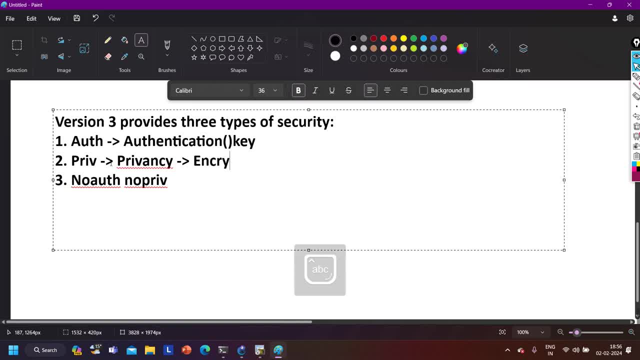 Privacy is nothing but encryption. Privacy is nothing but encryption. Privacy, Privacy means encryption. Fine, Now again, as you know, prev is not only encryption, But prev. It means authentication plus privacy, Authentication plus privacy, Authentication plus privacy. Getting my point, 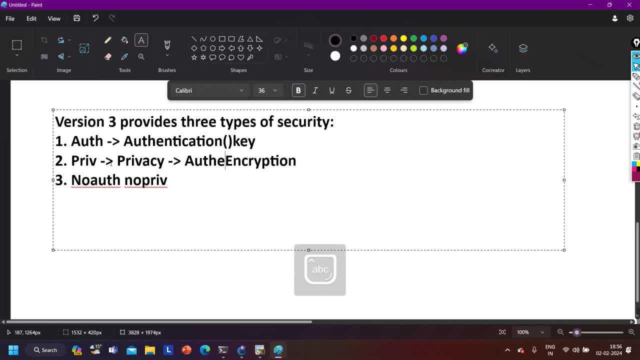 So you can see here authentication. Authentication plus privacy means encryption. Getting my point? So these are actually modes in version 3.. If you are using Auth mode means it will provide you authentication. So here you can configure what key. you can configure what key, right. 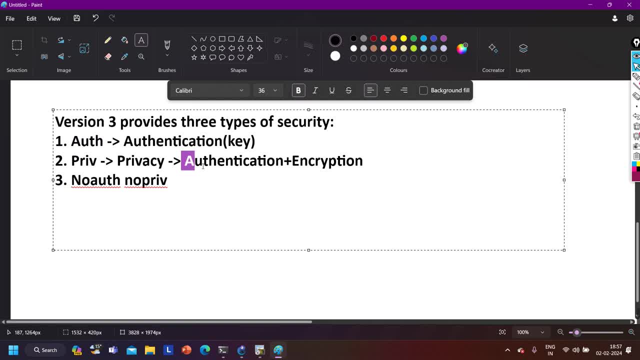 If you are using prev mode means it will provide you authentication plus privacy means encryption- authentication as well as encryption. So here you have to define authentication and encryption key Right. Again, we have multiple like algorithm for encryption, So we can use any one, like DS, 3DS, ES. 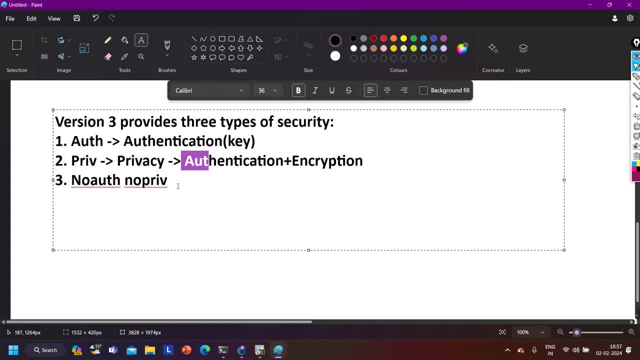 So we can use any one like DS 3DS ES. So we can use any one like DS 3DS ES. Fine, And no auth. no prev means SNMP, version 1 and version 2, right, Again, no security. 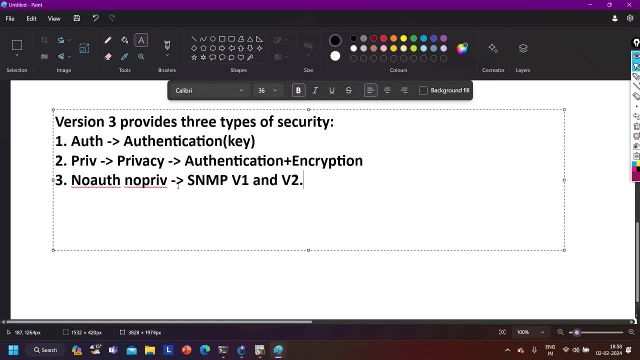 So in SNMP version 3, you have to define mode. If you are running SNMP version 3, you have to define mode and your mode can be auth prev and no auth. So in SNMP version 3, you have to define mode and your mode can be auth prev and no auth. 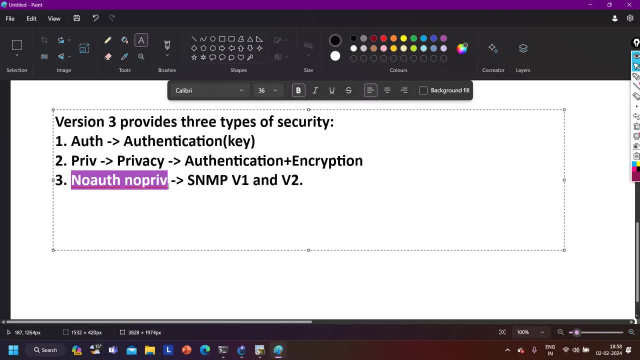 So in SNMP version 3, you have to define mode and your mode can be auth prev and no OculusIce Well, configuration, I will show you this, Don't worry. So if you want to understand as an mp configuration First, you have to understand as an МП deployment. 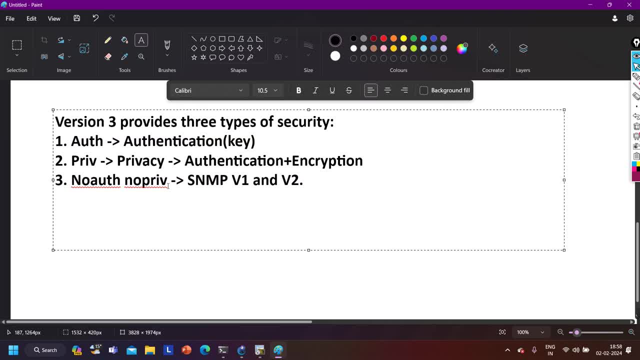 So now, guys tied to understand, there's an MP deployment. So now, guys tied to understand, there's an MP deployment. So till now, inversion three, What we discussed, what discuss? SNMP version three provide three types of security: auth, prev and no auth, no prev. 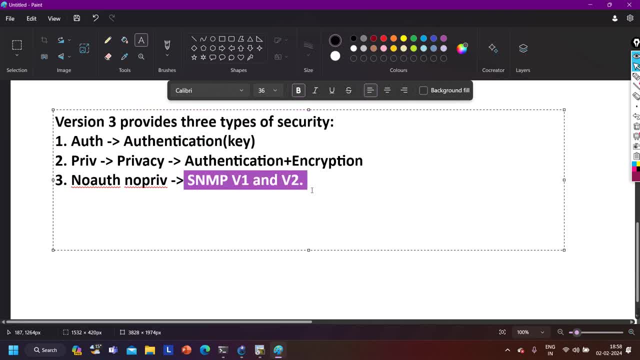 no auth, propanzu security like version 5.. prev and no auth, no, prev, Uh huh one and version two. prep means privacy. it is like authentication plus encryption, and auth mode means only authentication. you can define the key for the authentication. it will use that key to encrypt. 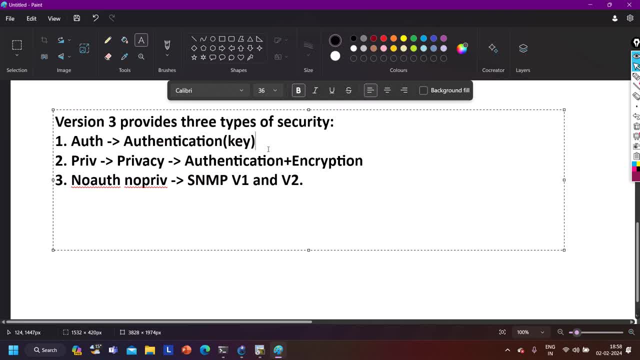 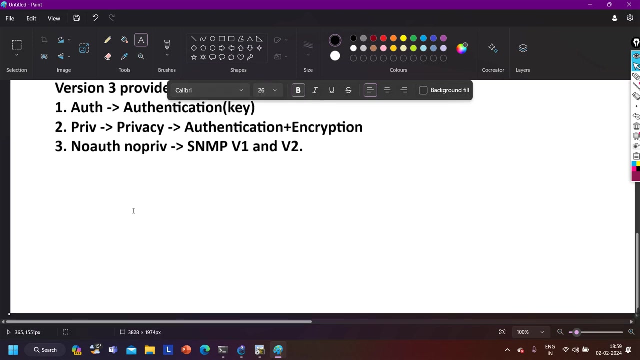 your data. that's it getting my point. it will use that key to encrypt your data. okay, now the very important thing to let me write here: to deploy SNMP, you have to categorize, categorized, your, categorize. I categorized your devices in term of group. right to deploy SNMP in your network, you have to categorize your devices in term of group, very important for SNMP deployment. 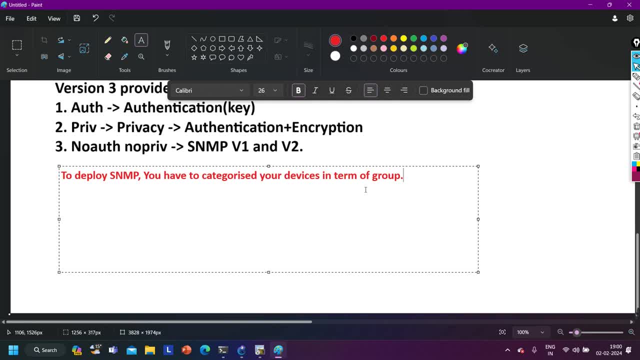 right to deploy SNMP, you have to categorize your devices in term of group right. let's understand with one example. let's say in my company there are some routers, there are some switches and there are some, let's say, any other device like, let's say, firewall. 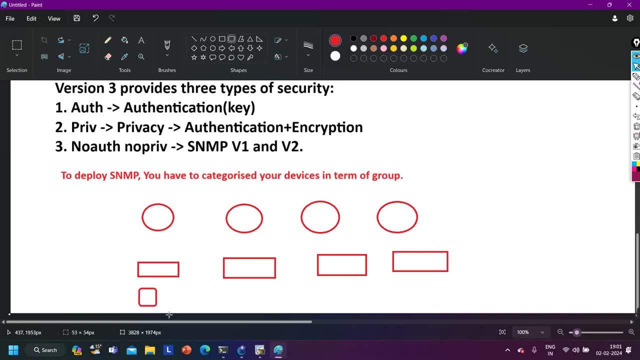 right. so i have some firewall as well here. these are, let's say, my firewall, getting my point guys. so to deploy snmp over here, first of all, what i need to do, i need to categorize my devices in term of group, how i can categorize all routers in a single group. 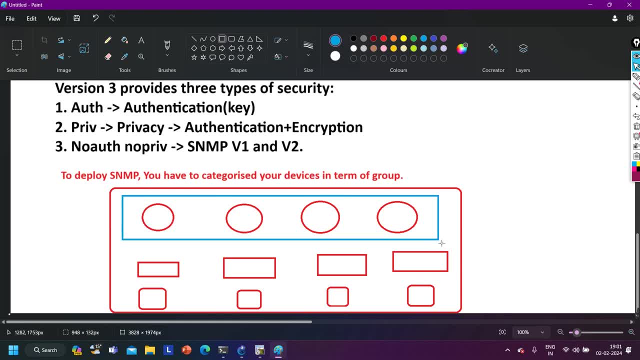 i can categorize all router in a single group. let's say i have categorized these all devices in a group and the group name for these devices is, let's say, group router, group group router. this is name of my router, is name of my group for these devices in the 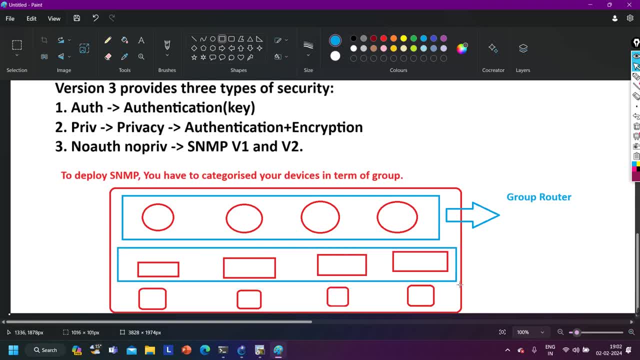 same way for switches. for these devices i have a group, i have created one group, and name of this group is: let's say what group: switch, group switch. and for firewalls, i have categorized these devices in a group and that group is known as, let's say, firewall group, firewall. 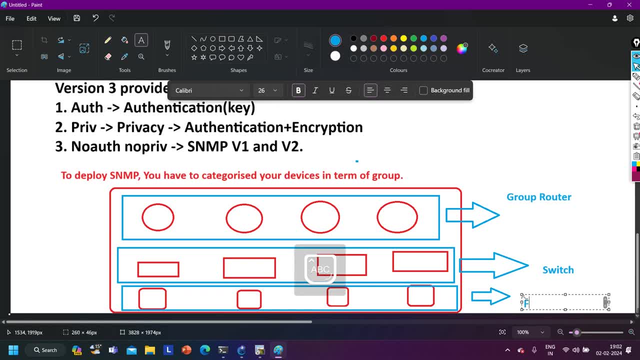 right. so in the same way, in real time, to deploy snmp, first you have to categorize your devices in term of group. so you can see, now in my company i have three group group router, group switch and group firewall. now i can deploy snmp over here. you know, now for each group we will create a username. 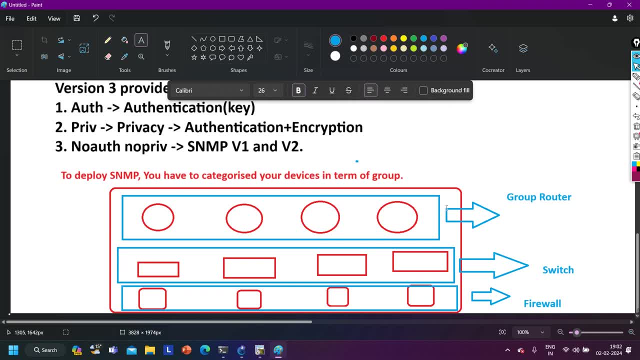 and password for authentication to authenticate the user. for each group, like for router group, i will create one username and password to authenticate the user. for group switch, i will create one username and password to authenticate the user. right in the same way for firewall also, i will create one username and password to authenticate the user. fine guys. 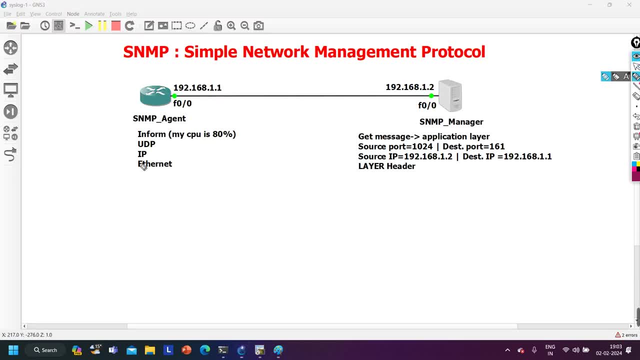 this is like you know. let's say, this is my scenario, in my scenario. you will never want that anyone who is connected in the network can get information of your SNMP, of your device or of your router. let's say, let's say here I am an employee of your company, right? so if I will install SNMP software over here and if I will? 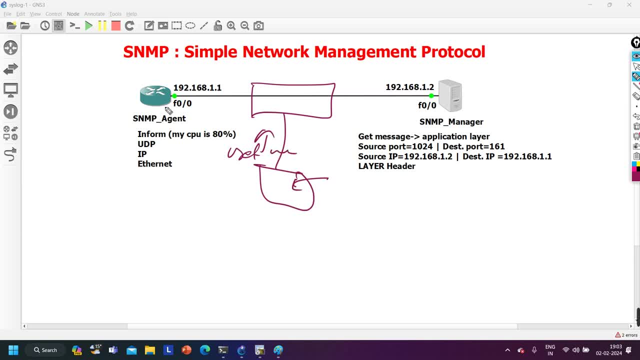 send what get message. get me version so your client machine can send me the information of is version to me as well. right? so first of all you have to authenticate the user that I am sending information to genuine SNMP server or not. getting my point? so that is the reason why. 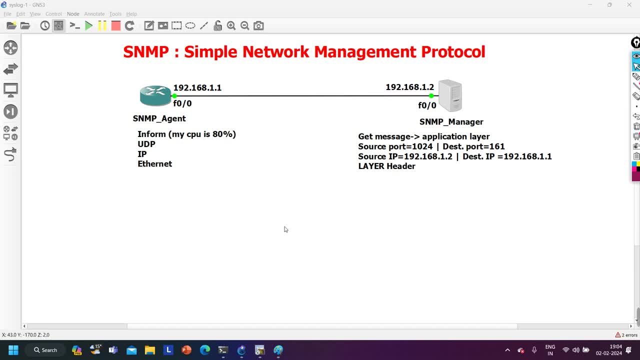 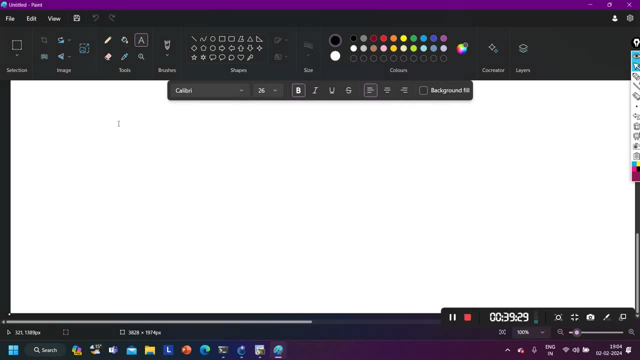 we come up with SNMP version 3 and nowadays, guys, we are using SNMP version 3. only fine, now let's move further. see the configuration. last part is the configuration part: how to configure SNMP in the network configurations. first of all you have to create: step 1, create access control list, access access, access list. right, what the 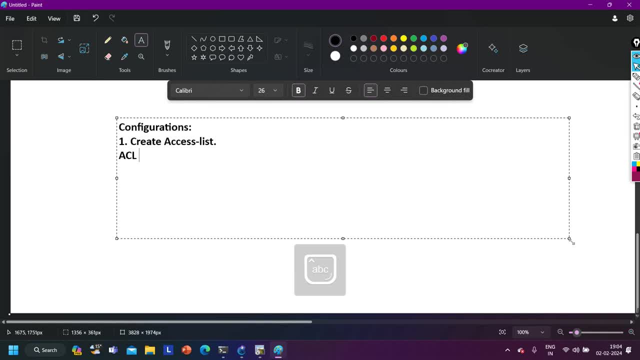 use of access list over here. so ACL or access list is used to define the location of SNMP server. so we will create access control list to define the location of SNMP server. who is your SNMP server? where is your SNMP server in your own network or it is in different network? getting my point? 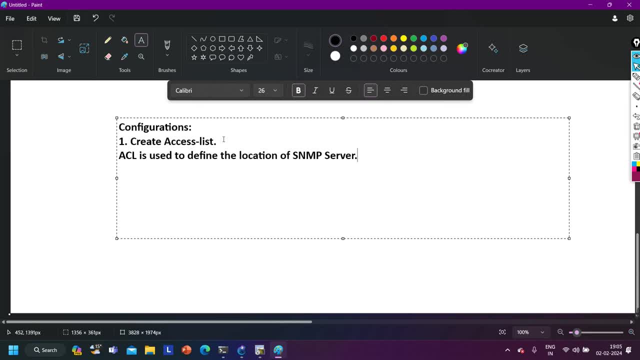 So here we are using access control list for classification of SNMP to classify the SNMP server or you can say to define the location of SNMP server. getting my point? So how I will create ACL may be. I can run this command: IP access list standard number. 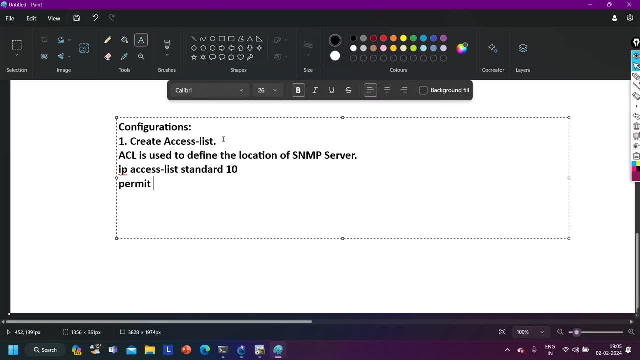 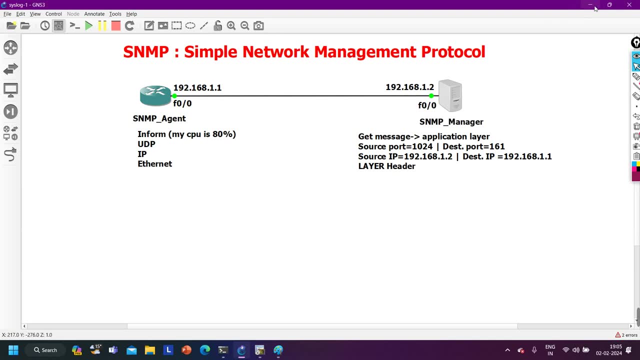 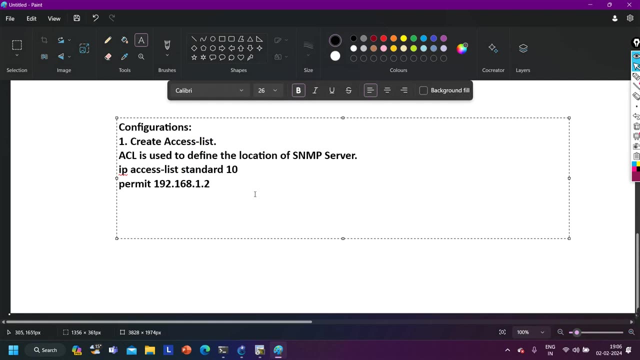 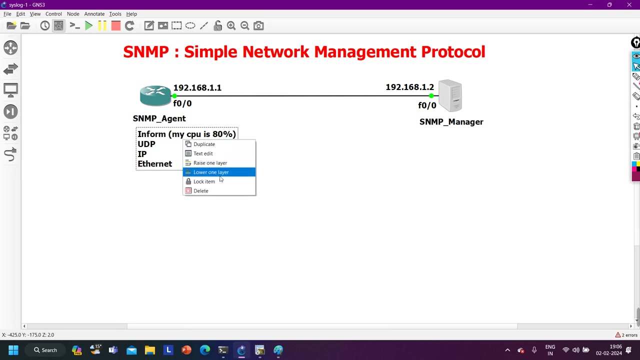 10, and then simply I can say: permit and IP address of my SNMP server. what is the IP address of my SNMP server? 192.168.1.2,, right, 192.168.1.2.. Let me do one thing. let me put this diagram as well here. 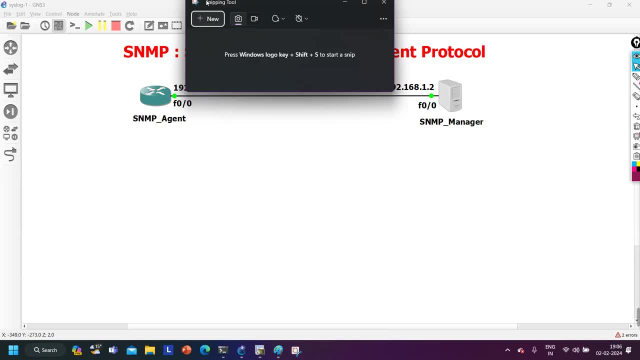 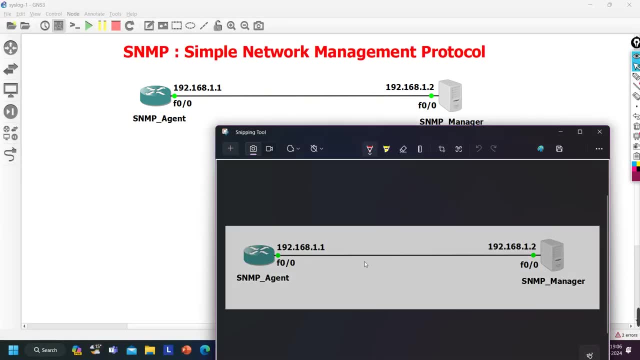 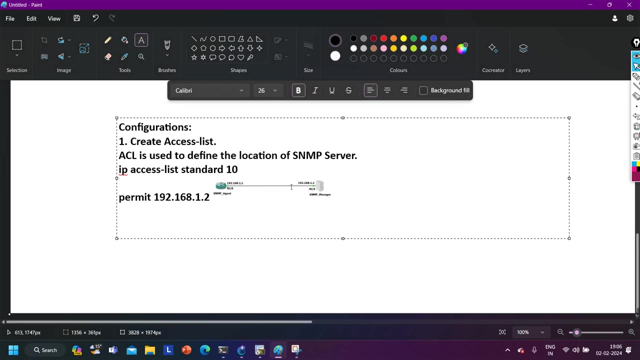 See So, So right. so on the client, on SNMP agent or client, I have first configured one access control list here. I have defined the location of my SNMP server. after that, exit, exit from here. then next step till now: we defined the location of SNMP server. now, guys, you. 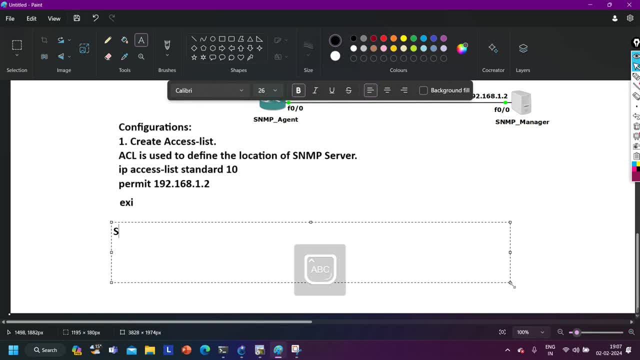 will learn next command. next command is SNMP server, SNMP server and then group. so on group, then you have to define group. so you have categorized your routers in a group and group name is router. so let me say router here. group name is what router and for this? 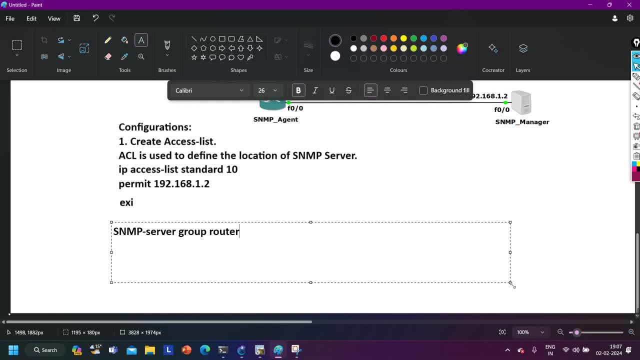 group, we will create one user name and password, getting my point. so next command will be to create user name and password right, first of all SNMP server, then group and then group name, after that which version of SNMP you want to use, let's say version 3.. 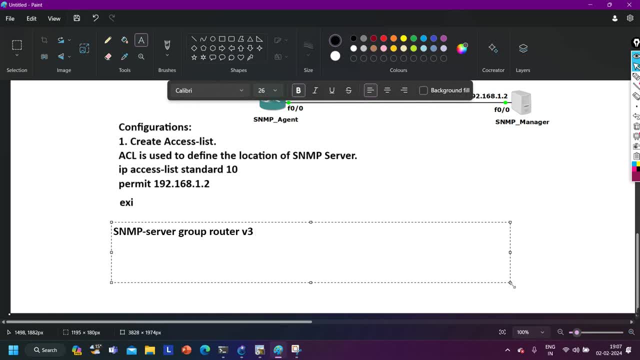 So I will define version 3 and then which mode? right. again, here you have three options: brief, auth and no brief, no auth, right. so let me use anyone, right. let me say what mode is what we can say. let's say brief, brief, right, and then we will call to access. 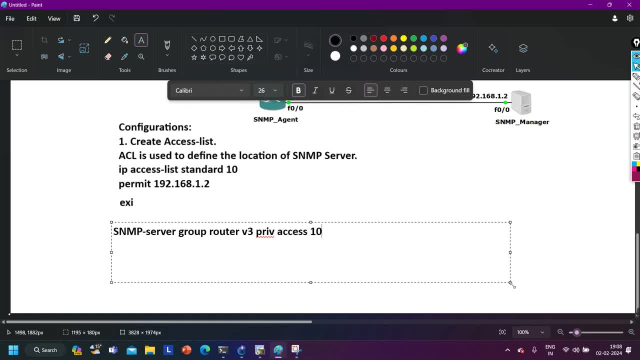 list: access 10.. Right, Then we will call to access list. so in this command, in this command, guys, what is the name of group? name of group: is router getting my point? what version I am using here? name. 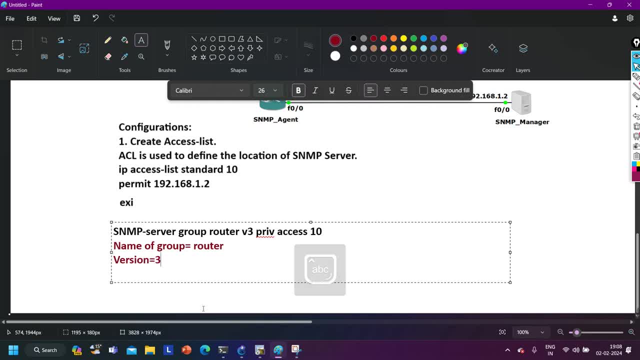 of group. is router, what version 3, version 3.. Then what mode I am using? Brief Brief means privacy plus authentication, encryption plus authentication, and then access control is location is location is of SNMP. is what ACL 10,. so this is my configuration getting. 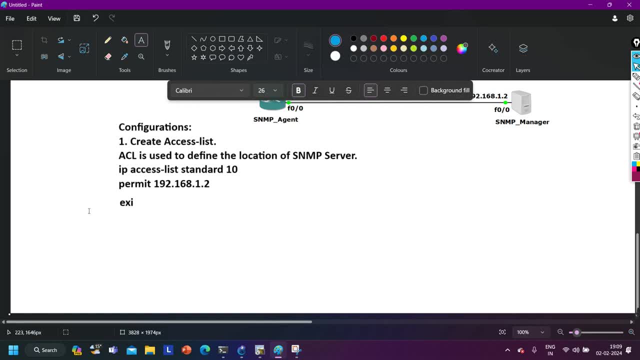 my point. Next one, this command over here. next command will be this one. fine, and hope this command is now clear to you. Then what is the next command? the last command. last command is this one last command is again SNMP. all command will start with SNMP, server, server, after that user. so, as I told, 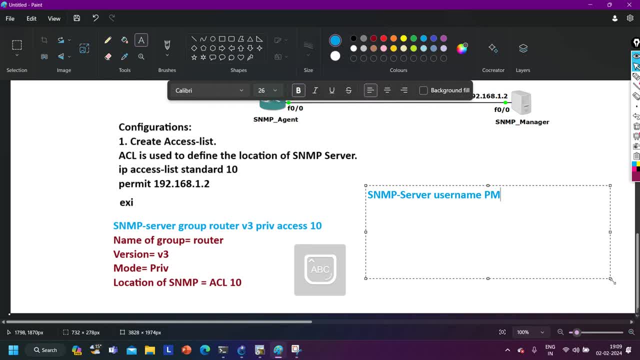 you. for each group we will create a user name and password. let's say user name is what pm? Then group name: For which group you have created this user name. so group name is router, and then what version you are using- version 3,, right. and then what authentication algorithm you want. 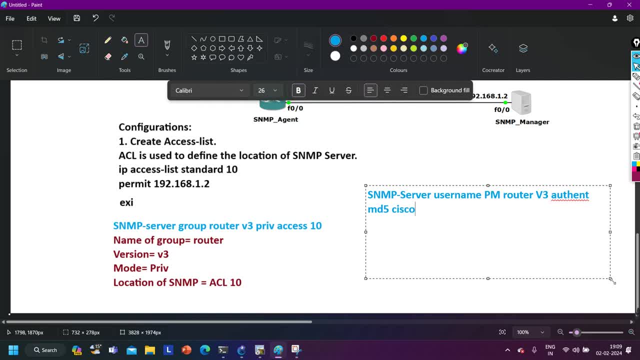 to use. let's say MD 5- and then what key you will use to encrypt the data. let's say Cisco, and then what encryption algorithm you are using. let's say 3DS or DS- anyone, you can choose 3DS or DS- and then what key you will use to encrypt the data. so let's say what. 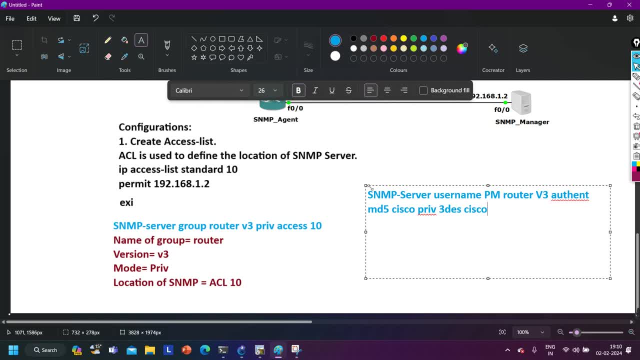 Cisco getting my point. So, guys, in this command- this is last command- in this command, what are the information? if I will talk about the information like user name, what is the user name for group router? that is pm, right. 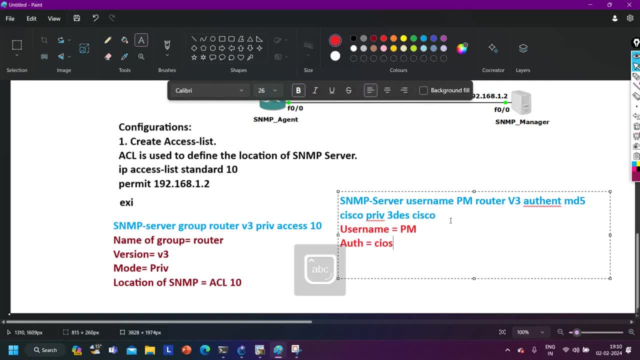 Then what authentication key I am using. I am using over here Cisco, Cisco right. then what DS algorithm I am using over here- data encryption, standard, Cisco right. and after that there is one verification command that is again very important, so you can run this command. 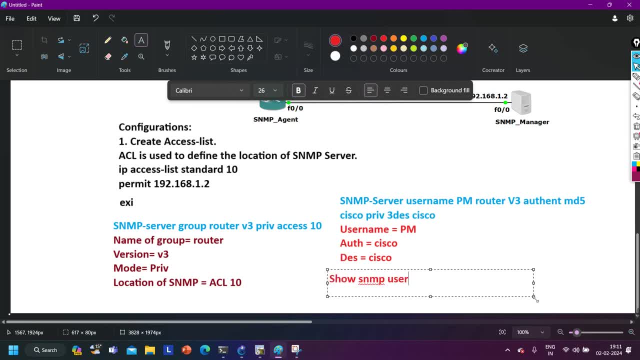 So snmp Right. So snmp user. and there are many more command I will show you while configuration. so hope configuration is clear to you, right? So this is all about the theory part. in theory part, guys, we discuss messages like set message. 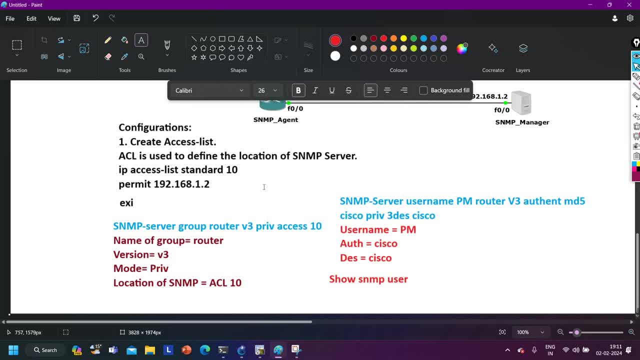 are used to apply configuration like: set IP, set VTP domain name on switch, set host name, set banner, set IP address right and manager will always use this message and it will send on port number 161.. Then we have get message to gather the information. to gather the information and again get message. 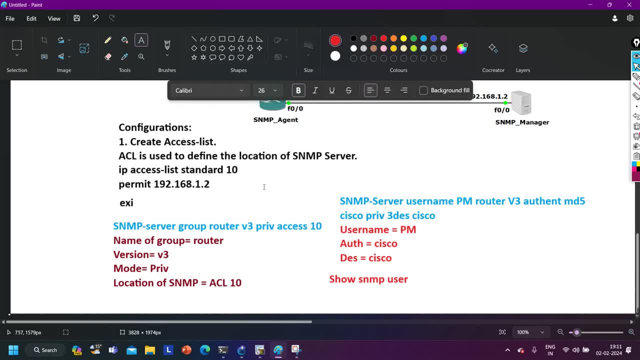 will be sended by snmp manager always. then we have trap message right for the condition and trap message will be forwarded by client to server on port number 162, right. Generate a trap message whenever a VLAN is created or deleted on switch. 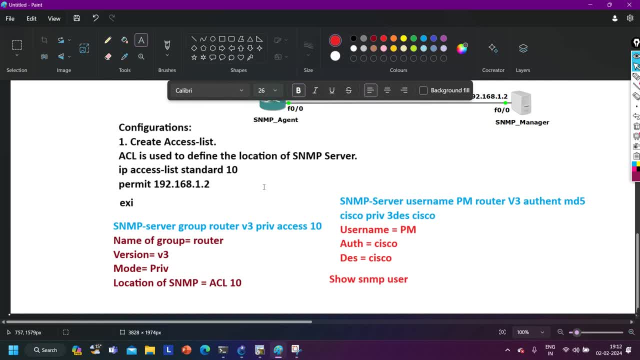 So these are what conditions. so, whenever someone will create a VLAN, it will generate, it will, trap message. whenever someone will delete the VLAN, it will, your device will generate a trap message, right. So now here, let me show you the configuration. same configuration I am going to show you. 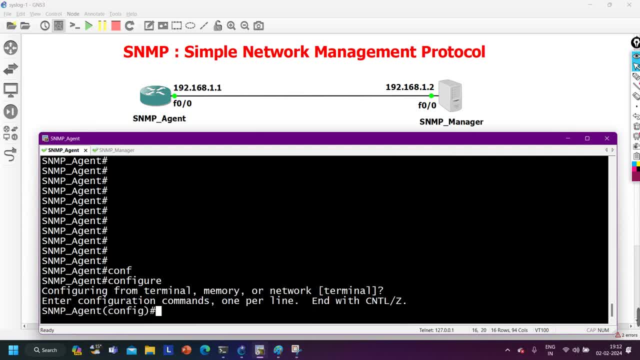 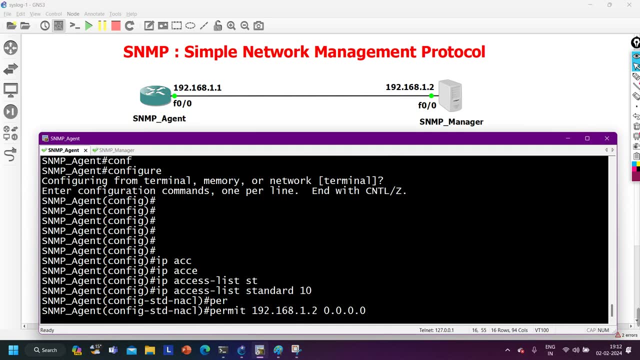 over here on snmp agent machine. So go to config mode. first of all you need to create what access list. so let's say IP access list, standard number 10, and I am going to say permit 192.168.1.2, right, 0.0.0.0, fine. 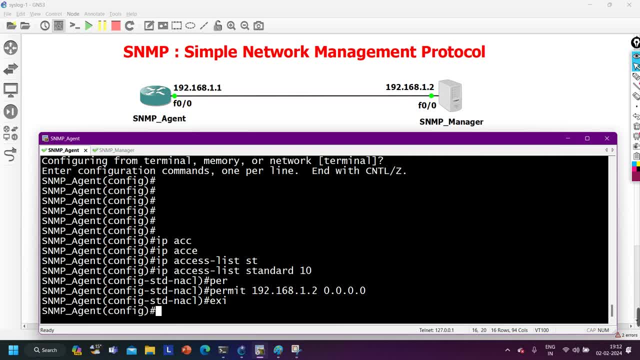 then exit. This is for defining the location of your snmp server. after that snmp server, snmp server and group group name. let's say group name is router. right Then, guys version. if you will put question mark, you can see you have three options. 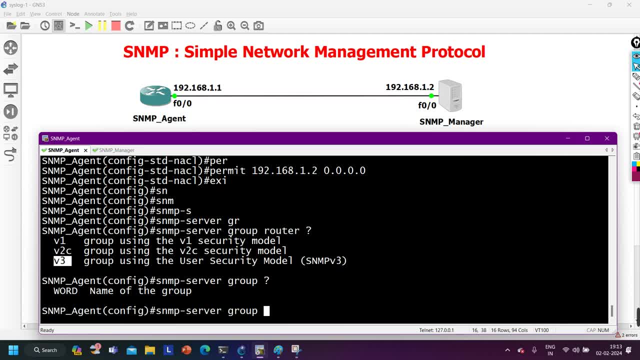 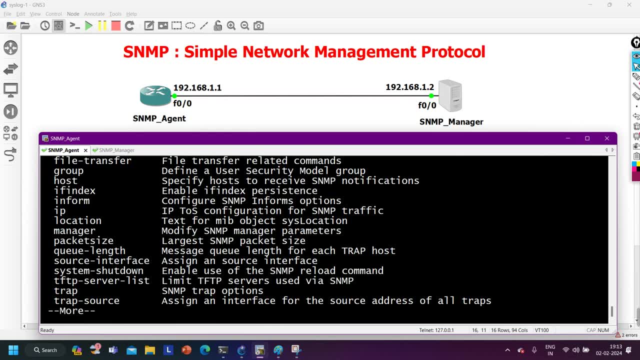 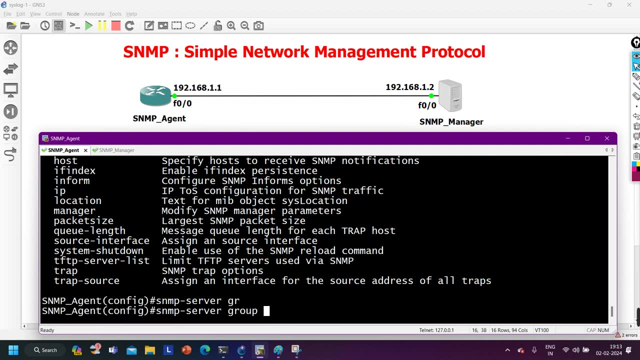 version one, version two, version three: Before this: if you will put question mark over here, you can see it's asking for the group name Before it. if you will put question mark, you have multiple options, right, So we can't discuss. you know these all over here in a single video, right? but the important 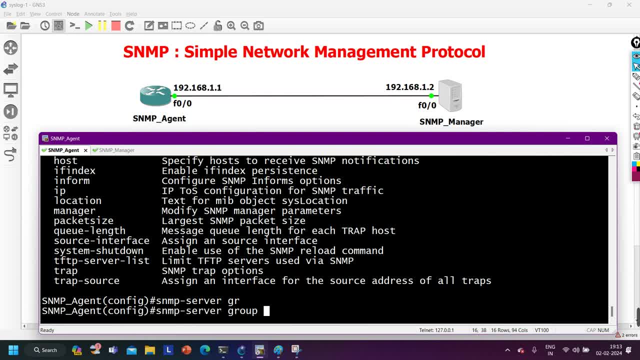 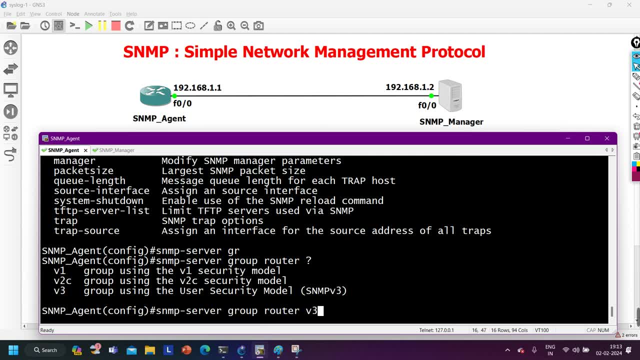 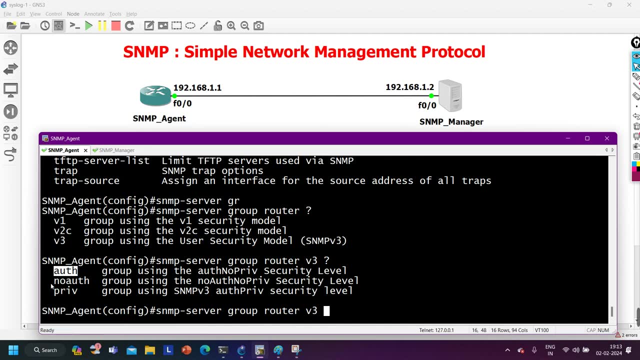 part I am discussing over here, like snmp server group and then group name, let's say router, We will define the version. let's say version three, yes, version three after that mode. So see, you have three mode: auth mode, no auth mode, this is no auth, no prev and this: 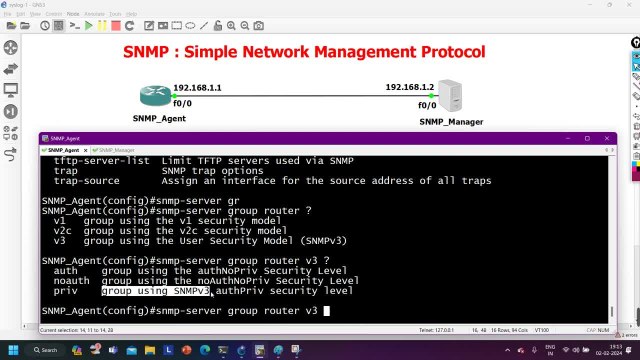 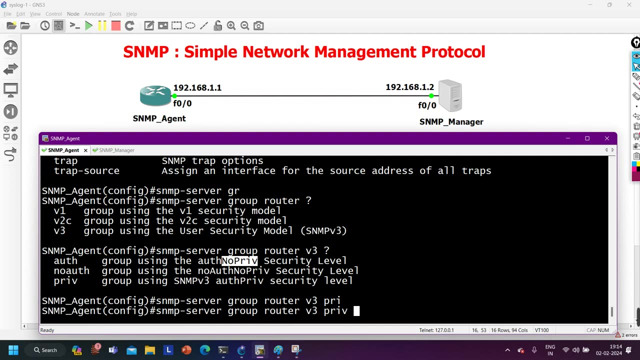 is prev mode: Group using snmp version three: auth prev security label. auth means group using auth, no prev security label. Right Only authentication, no privacy, no encryption. So let's say I want to use what prev mode I want? authentication as well as privacy means encryption. 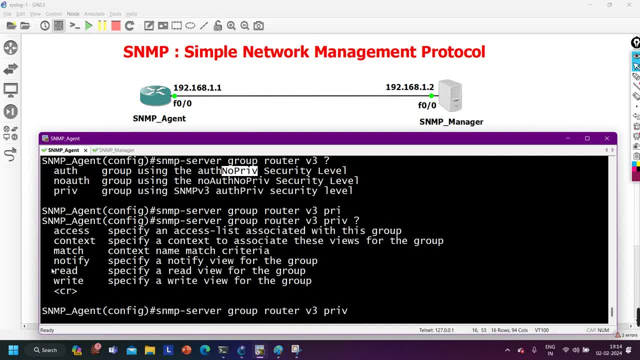 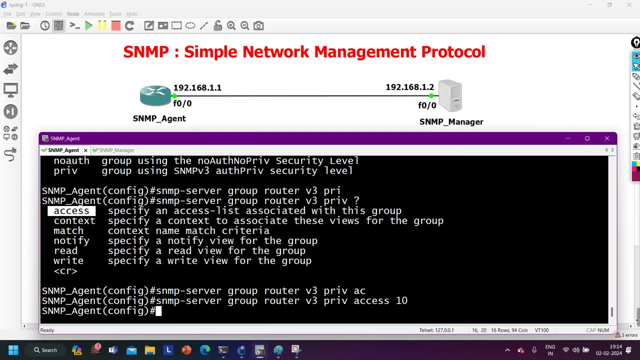 So I will use which mode? Prev mode, And then I will call to my access control list. access list, access list number 10, right, This is command, right guys. So here the name of group is router, version is three. mode is prev. 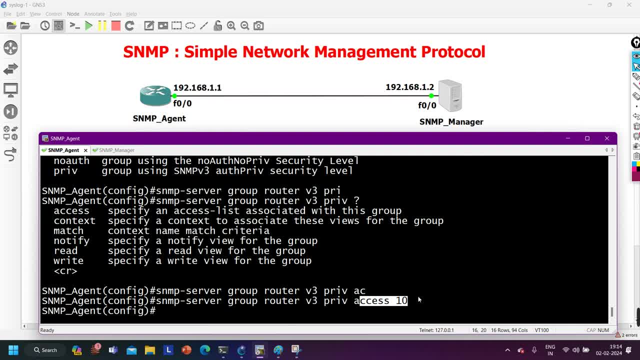 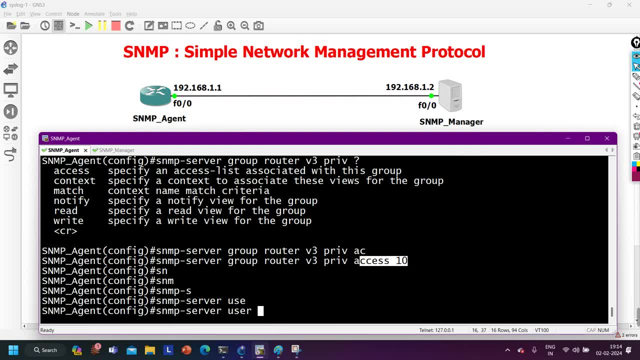 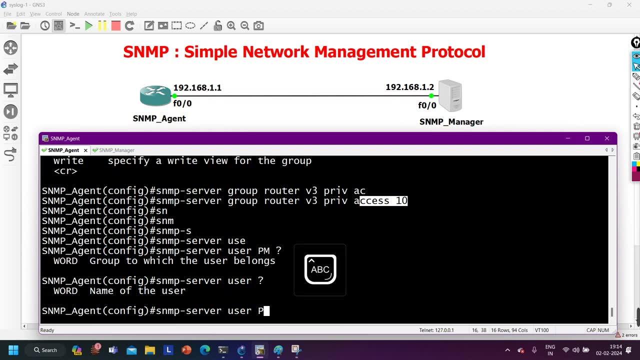 The device location is access list number 10.. The next command again snmp server. after that username. Username is what PM? For which group? For which group? Here you need to define the username. So username is PM and then for which group you are creating username. 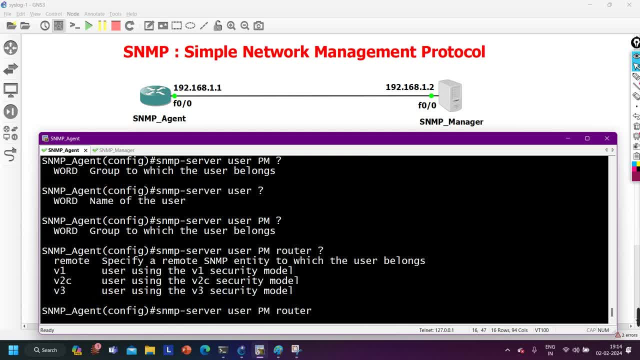 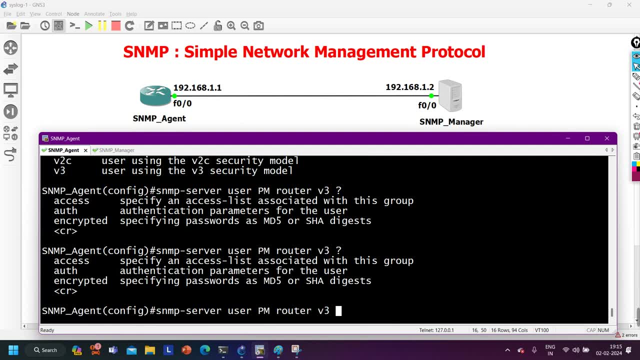 So let's say: for router, for which group? For router, Then what version you are using, Version three, Then See Authentication, encryption, Right? So same command, same this command you are running here, right? So let's say: authentication algorithm is what? MD five? 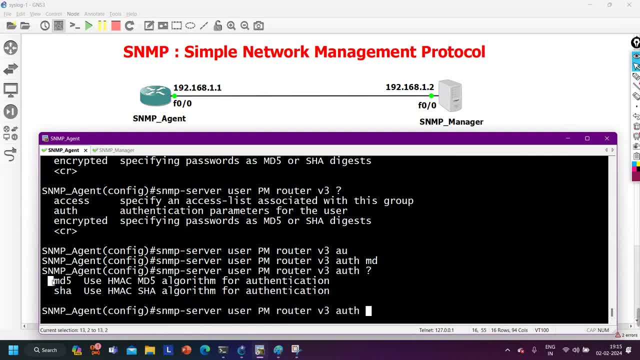 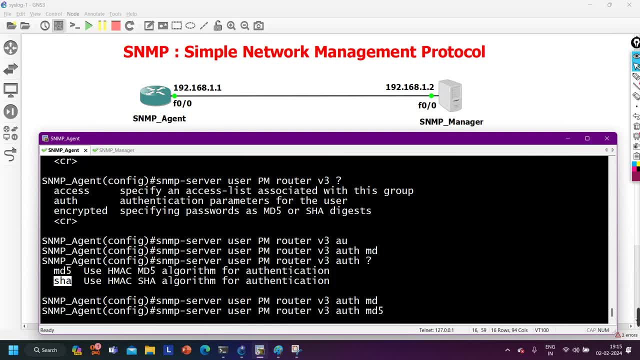 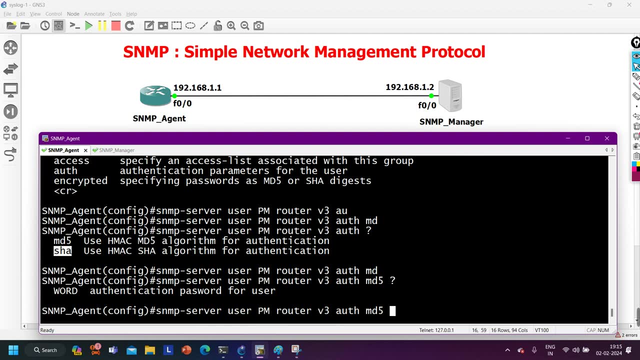 And if you will put question mark here for authentication you have. you can see two algorithms here: MD five and SA, So you can use any one. I'm using MD five over here Then for encryption right now. first of all you have to define the key over here, right? 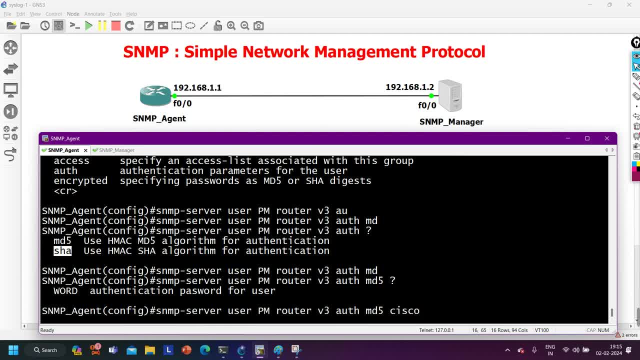 What key it will use to encrypt the data by using MD five algorithm- that is Cisco. What key it will use to encrypt the data by using MD five algorithm- that is Cisco. So actually, what will happen? It will kick, you know, generate one hash value by creating with the help of this key. 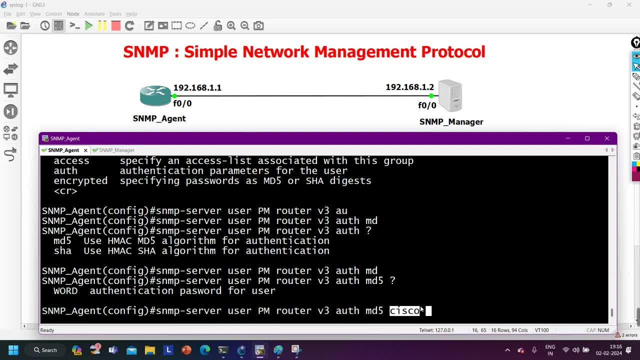 with the help of Cisco. It will generate one hash value with the help of key Cisco And on the server, whenever you will, you know a set set message or get message or any message. you have to provide these all information, like key target IP address right. 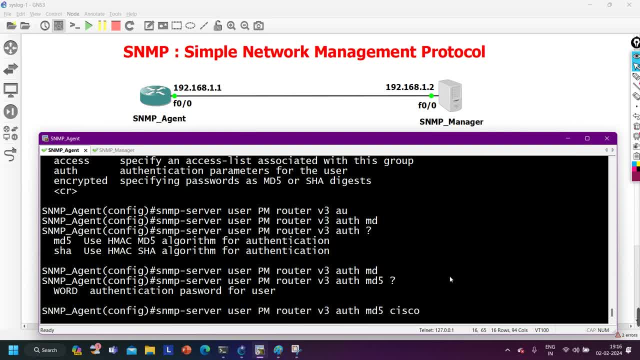 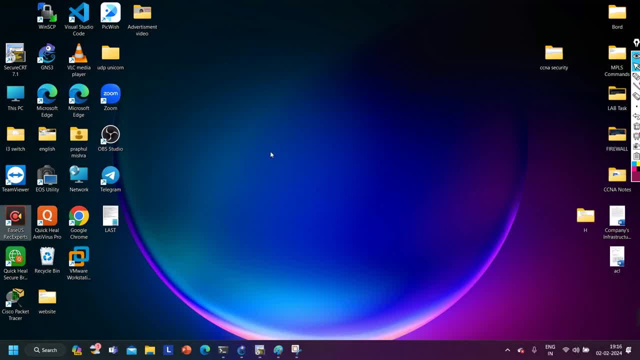 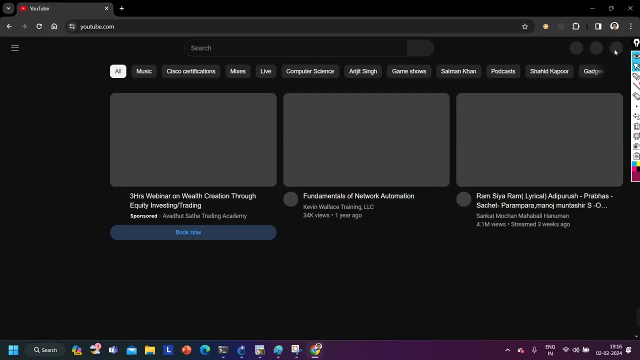 Then only you can get information or you can apply the configuration right on the devices. So if you don't know how to configure it right, I have already one video guys on SNMP Where I have performed the practical in packet tracer. So if you want to watch that video let me show you right. 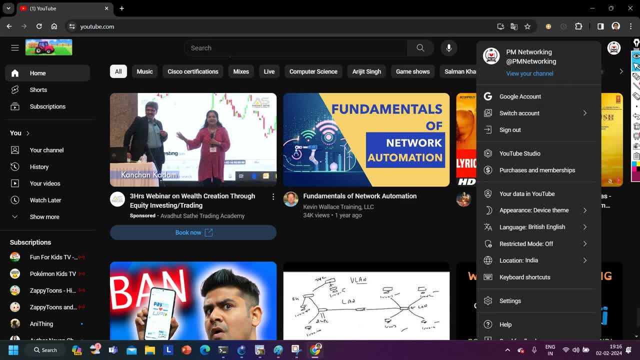 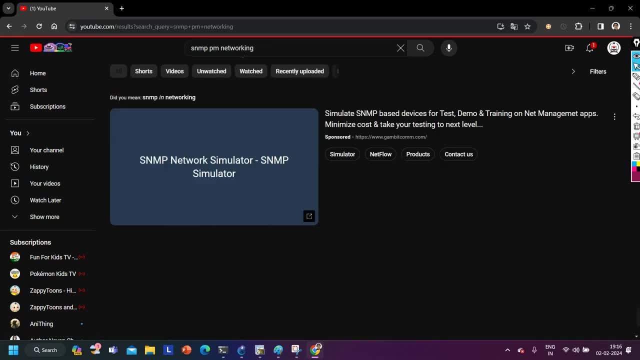 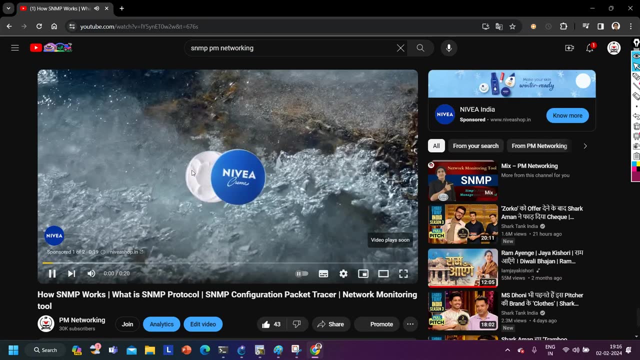 In that video actually, you will get the SNMP server configuration. You will get SNMP server configuration, SNMP PM networking. So this is the video, this video- I'm talking about this video to see in this video. in this video we have configured the SNMP server configuration. 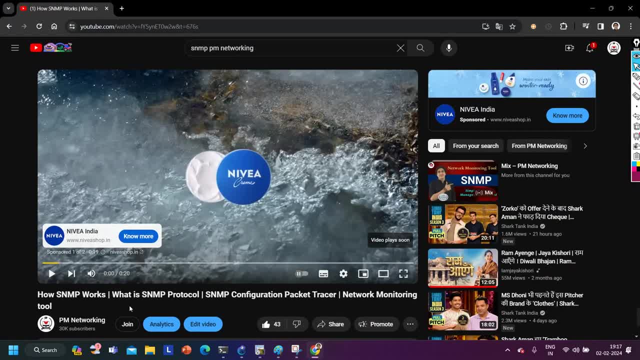 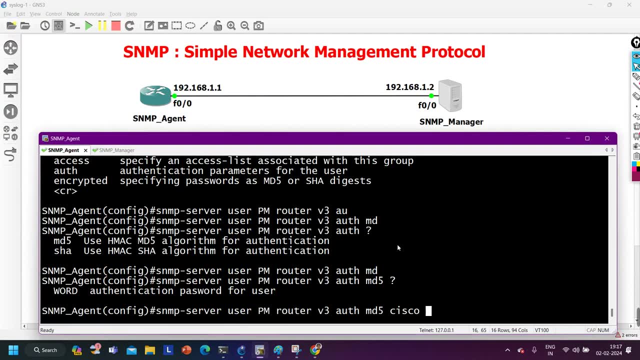 Okay, In packet tracer, right? So you can see the title. you can search it. If you want to know how to configure SNMP server, here we are. we are just configuring SNMP client device, and this is only important for you as a network engineer, right? 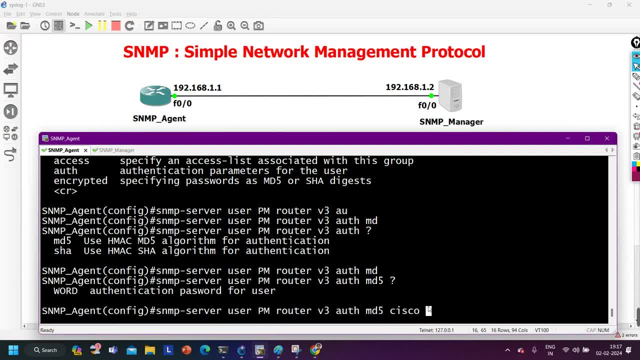 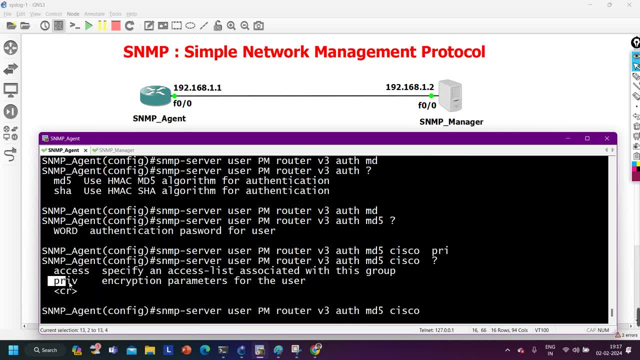 So, guys, authentication algorithm is MD5 and key is Cisco. Now I am going to define what encryption means. brief, right, And if you will put question mark here, you can see you have only this option. So we can. you can call to access control list here, right? 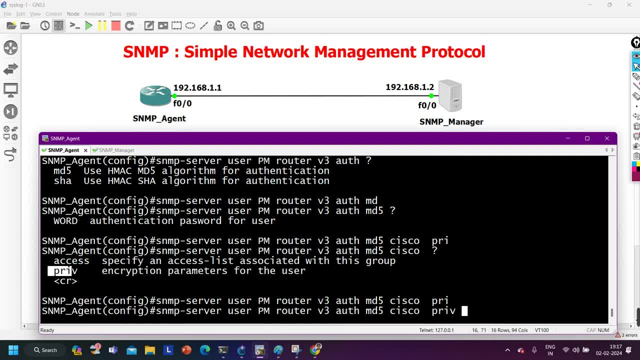 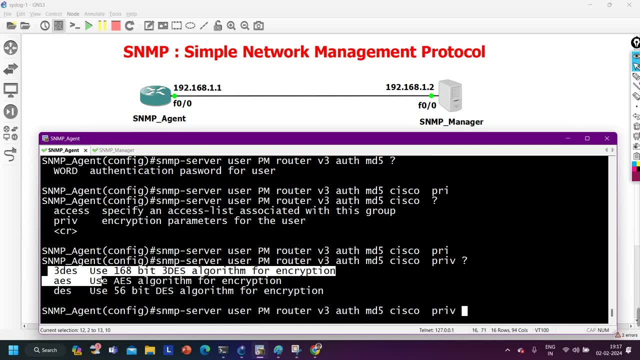 So let me say brief And then what encryption algorithm you want to use: DS, 3DS, AES. So let's put question mark over here. You can see we have three options, right: AES, advanced encryption standard, data encryption standard and thrice or triple DS. 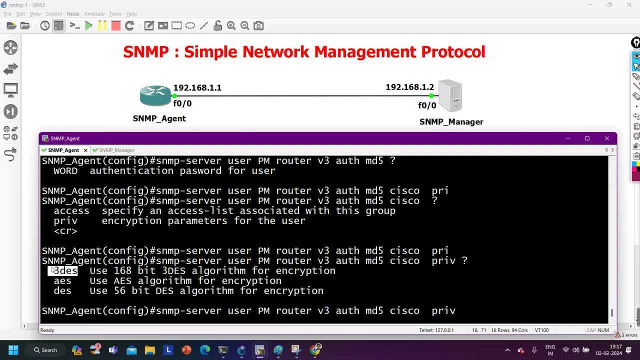 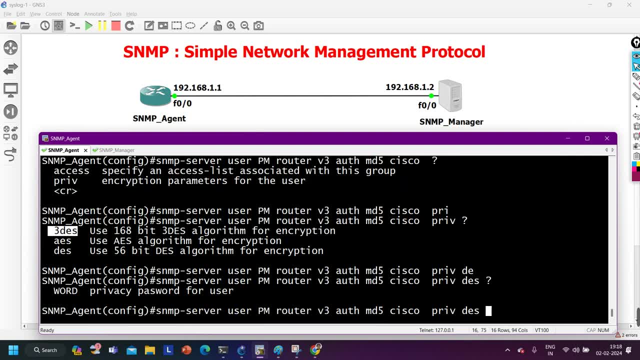 That both are same. It will run DS algorithm once And this algorithm, 3DS, will run Same. run same algorithm, thrice, right? So let me use what DS over here, right? And then what key you will use for encryption, let's say Cisco. 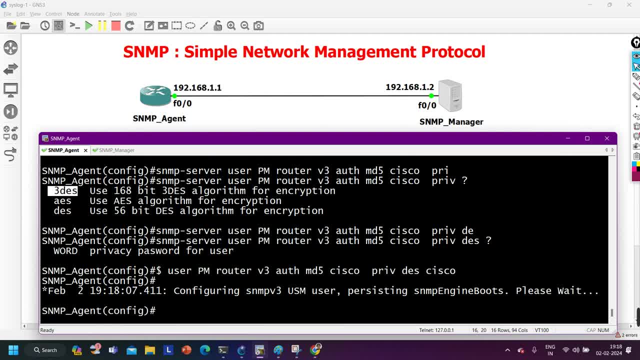 This is the configuration of SNMP guys version three, right? So now you can see the log message as well, right? Fab two, this is the date and time. then configuring SNMP version three user. Leave this message. This is not important for you now, right? 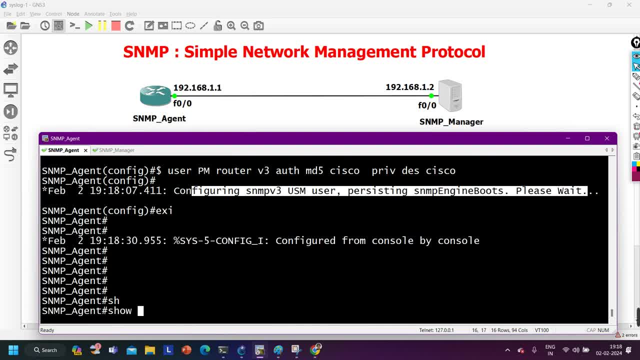 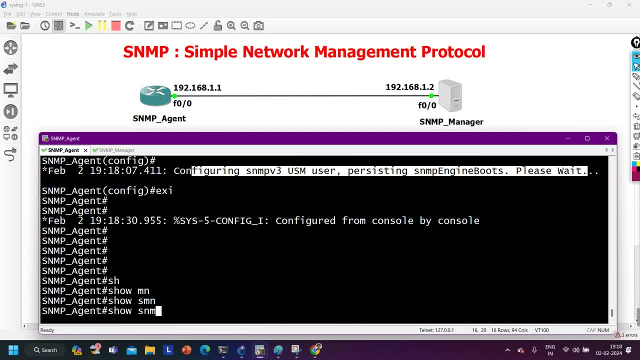 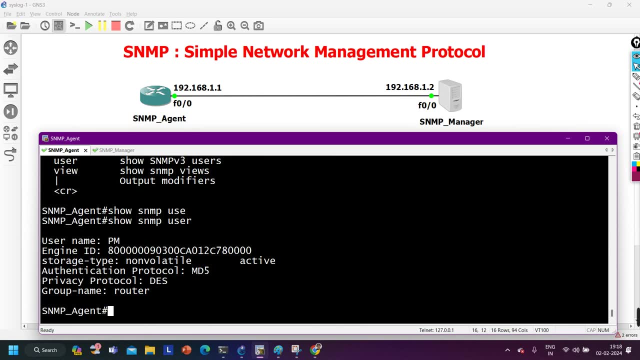 Again, this is important, but not for now. Now, what command I can run here? So SNMP, SNMP, sorry, So SNMP. and you have multiple options, Like if you want to check users so you can see you have only one user. username is PM. 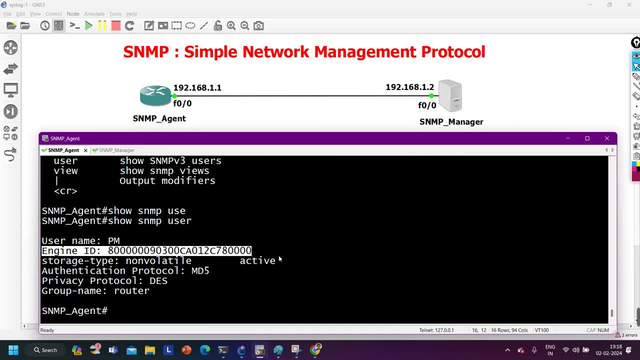 right Again, there is concept of engine ID guys in SNMP. You have to learn it. You can check book or you can Google it, right? If you want to learn all about SNMP, definitely you have to enroll for paid course, right? 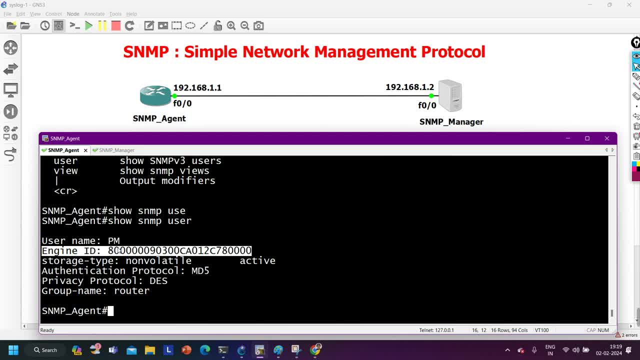 Because in one hour or two hour we cannot cover entire things of SNMP, right? But, guys, these are important and these topics are in your syllabus, right? So I have covered all topics, which is in your syllabus, right? 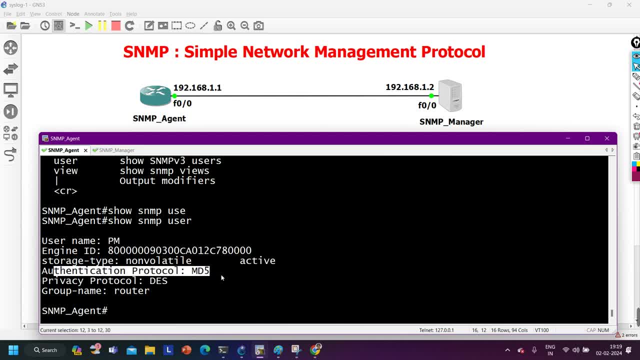 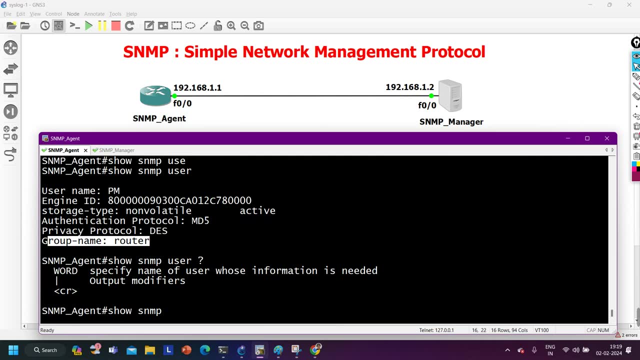 So you can see here: Leave this engine ID for now. right, See, authentication protocol that I am using is MD5, encryption algorithm or protocol that I am using is DS and my group name is router. Then is there another command, Not here. 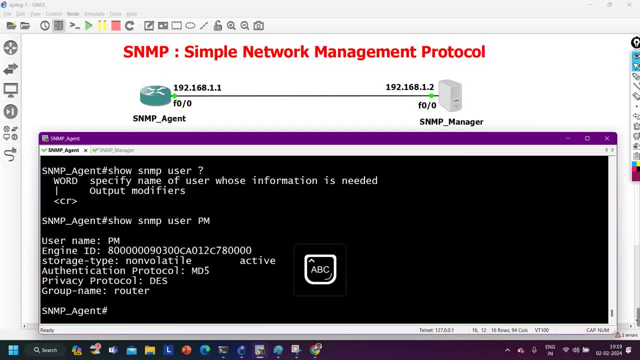 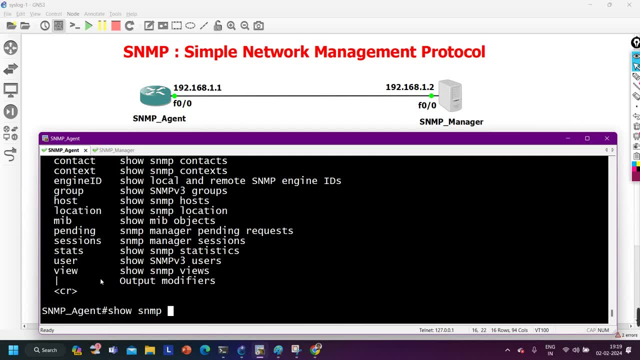 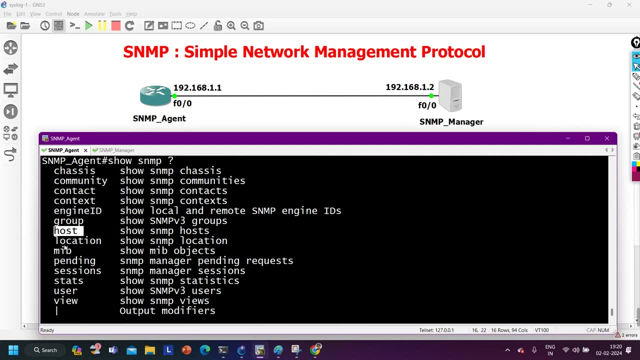 Here what we can do. you can put the username as well, Like, let's say, if you have multiple users, so you can find the configuration with the help of username. also. After that: Okay, Group host. we can say what location? okay. 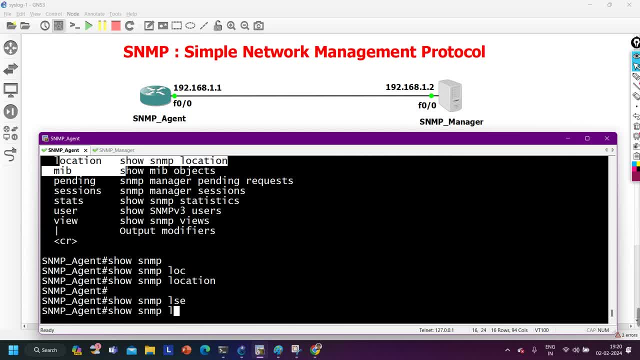 So it's not showing sessions, So we don't have any session till now. Okay, Leave it for now. Okay So, SNMP, SNMP, what we can say, Okay, Okay, Okay, So I have my OSD, since I got the data. 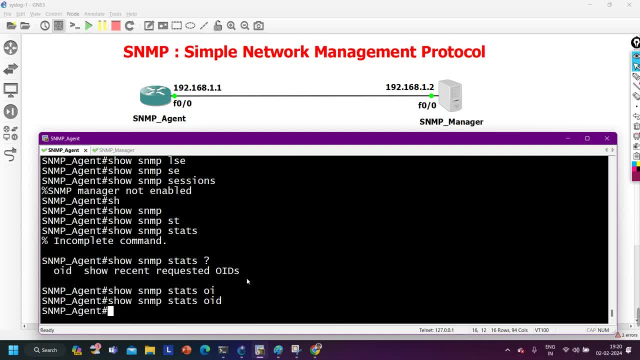 Okay. So if I get check OK So we can say we can write a status ODI. You know what is ODI? ODI is very impotent object identifier. You know, on router or on your switches, every features on the devices have ODI. 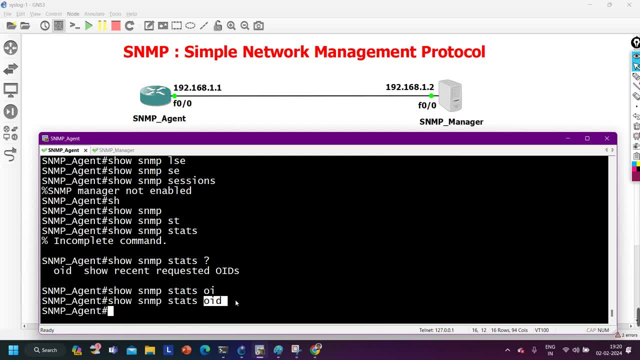 All the features. are you sorry, guys? in the simple word, what you can say, every features on the devices is identified by ODI. let's say you have a feature- EIGRP, OSPF, BZP- that you can run on routers, so those features will be identified by ODI. 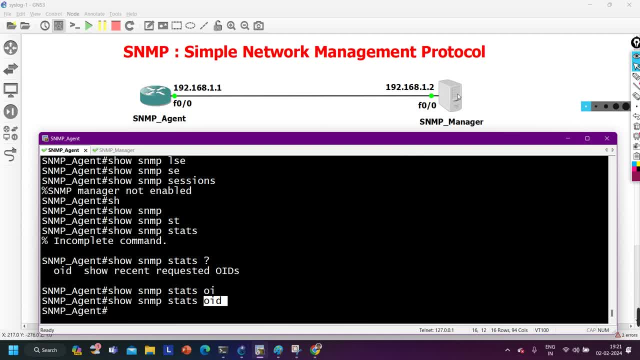 so let's say, if this router will get one get message from SNMP manager and in that get message, information is get me the IP address of interface. so for the IP address, device will have one ODI through that we will identify the services, features, object: identifier. so my device, my client or agent, your router switches. 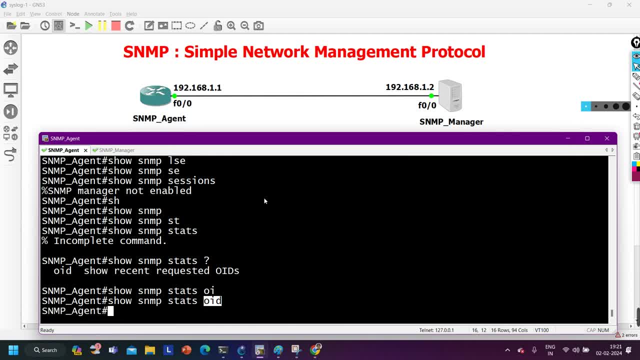 will send that get message to your ODI. to which ODI? to the ODI associated with interface, or if you are getting message for hostname. so again for hostname. hostname is also one feature. for hostname, we will have one feature, we have one ODI.